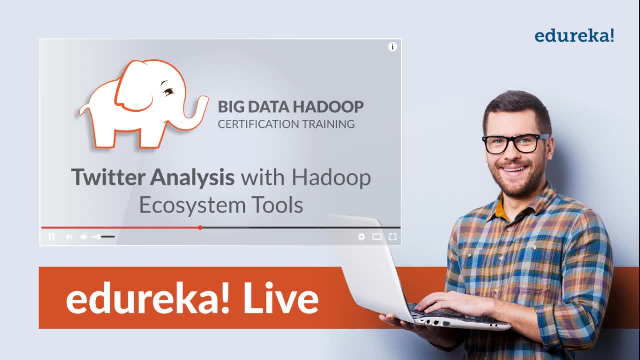 Hello and welcome everyone. this is Reshma from Edureka and I'm very excited today to take up this live session on Hadoop. So we're going to do a Twitter analysis today using different Hadoop ecosystem tools. So, without wasting any more time, let me tell you what. 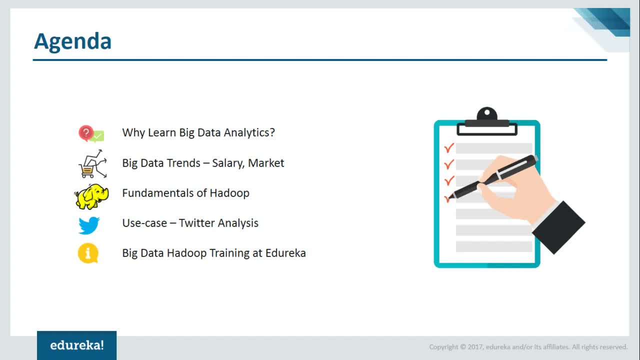 this session will cover, because I don't want to hold you for much longer, because it is Friday, So here is the agenda. So at first, we'll learn what is the need to learn: big data analytics. Why am I talking about this particular technology? And in order to answer, 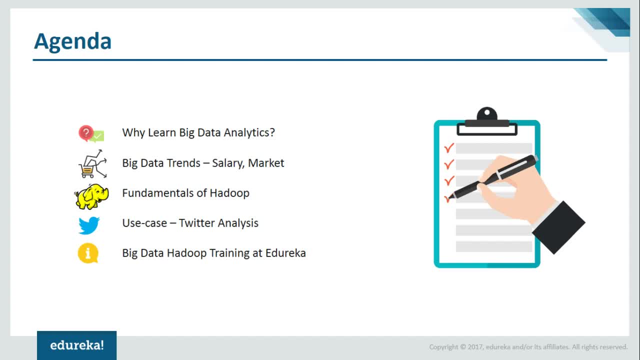 this question. I will be telling you the big data trends, the salary you can expect as a big data professional and what the market holds for this technology. Then we'll move on to understand some fundamentals of Hadoop and we'll put all the fundamentals into use. 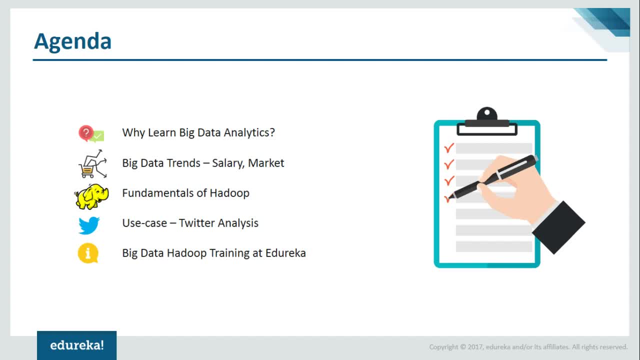 where we'll be doing a Twitter analysis. we'll be doing a sentiment analysis to find out how popular is big data and Hadoop, And also I'll be telling you about the big data and Hadoop training that we have at Edureka, where I'll be explaining you the entire course. 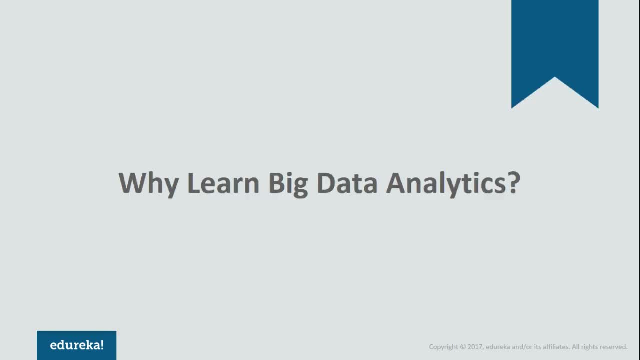 curriculum. So let us get started. So the first topic is: why learn big data analytics? Now, there are numerous reasons because of which different organizations and people are going in for big data analytics, And I have tried to list down the four most obvious reasons. 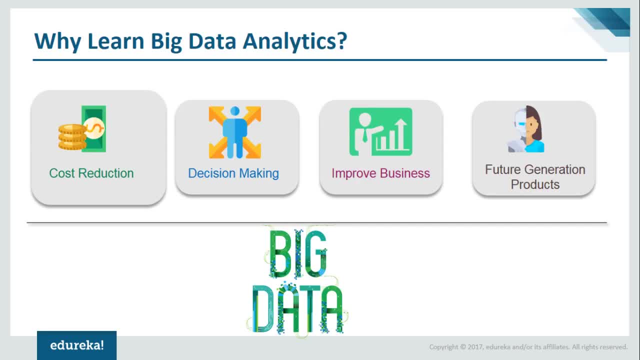 which, according to me, is because of which people are taking big data analytics. So the first is cost reduction. Now, when you analyze your data, you will gain a lot of insights and you'll find out different ways on where you could save your money on. So hence big 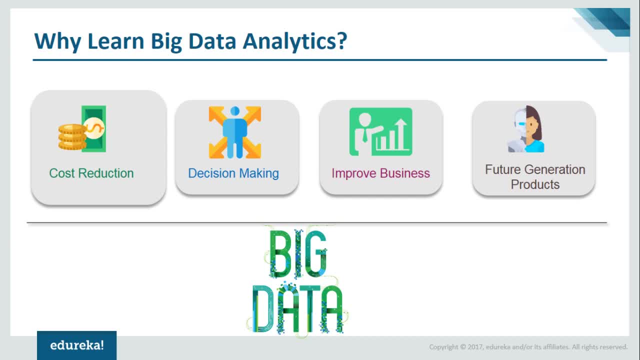 data analytics can help you to save your money And also it can reduce the total cost of ownership of your organization as a whole. The second: it helps in better decision making. How? Because when you analyze your data, you can see that the cost of the organization is lower, and 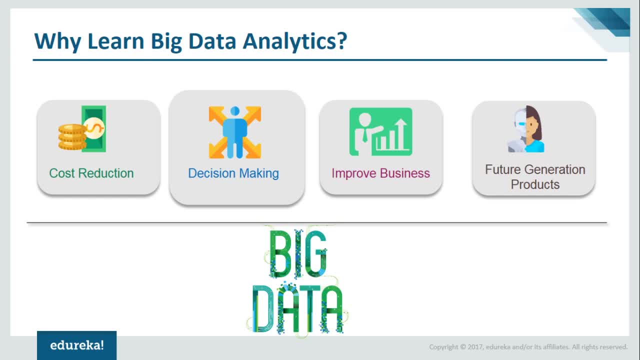 the cost of the organization is higher. So, when you analyze your data, you'll be somewhat able to predict that what is going to be the outcome of implementing something, And hence it will help you to make a better decision, because if you already know the result, how? 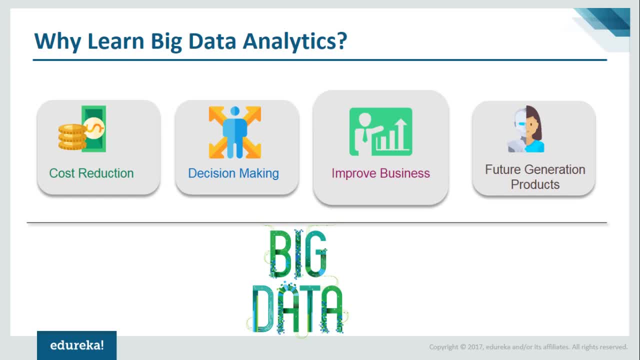 hard can decision making be right. It will also help you to improve your business because with the insights that you'll get by analyzing data- you're analyzing your organization's data- you'll be able to figure out that how can you implement your business strategies. 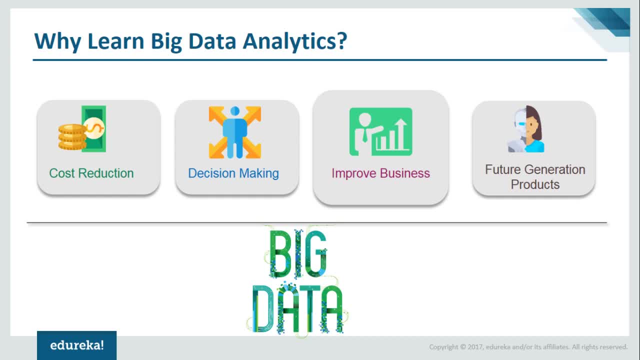 more effectively by cutting out both costs and costs. It will also help you to understand your target audience better and improve your business. And now let us talk about the future generation tech product that is believed to be a part of everyone's day to day lives in future, Something like self-driving cars. How do you? 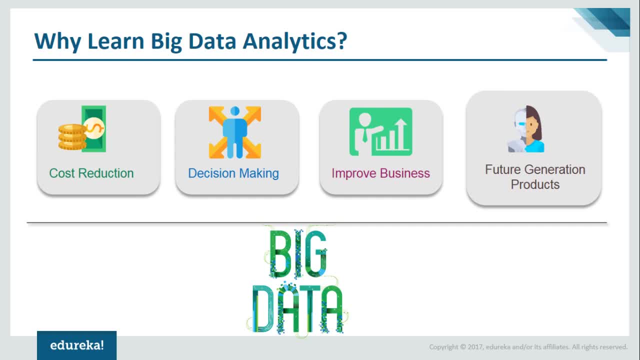 think a car drives on its own. It has to analyze all its surrounding data, which is a lot of data, let me tell you- because it has to predict that, what might be the possible obstacles that might come on its way, And it has to halt. 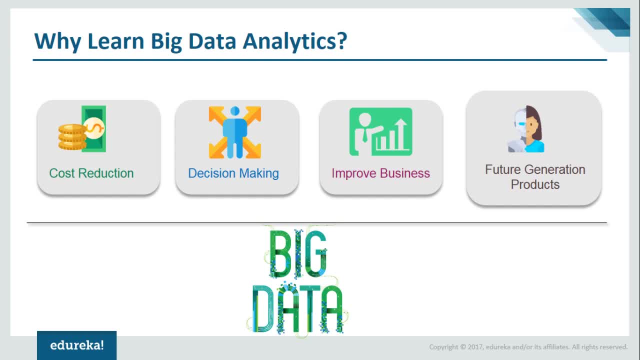 Let's talk about smart devices, Internet of Things. How do you think these devices are getting smarter every day? It is because they're getting trained on a lot of data, which is nothing but big data. So these are the various reasons, the four most obvious reasons which. 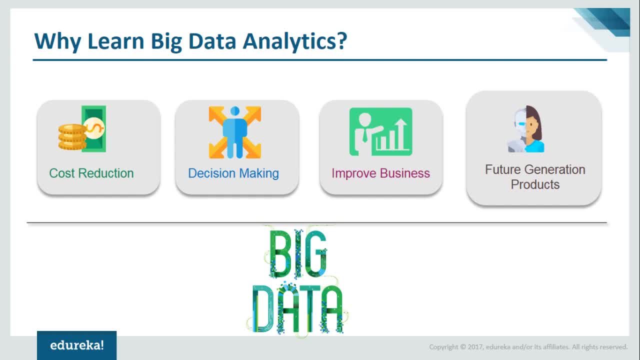 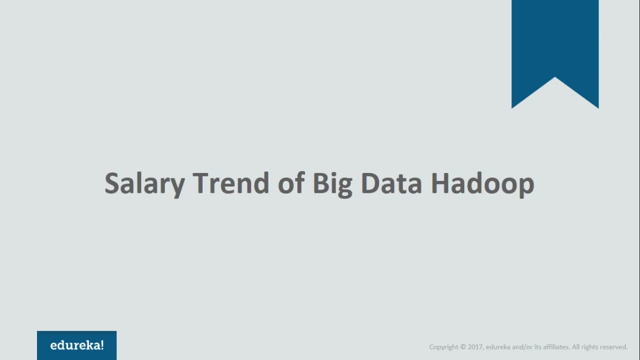 I think, why big data analytics is getting popular every day. And now let us talk about the actual reason for which we want to learn big data: because we want to excel in our career And we want to grow and learn more skills And, of course, we want to earn some money. 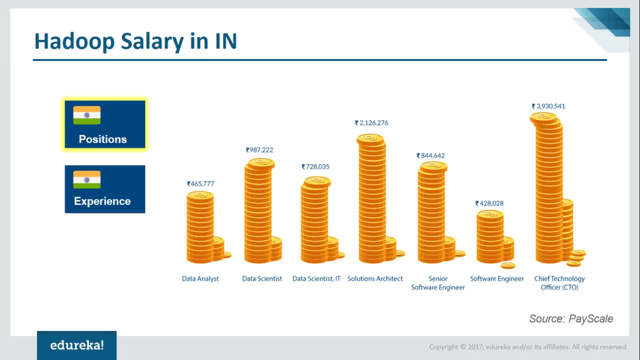 So let us see the salary trend of big data. So these are some of the indicative figures that I have collected from PayScale. Now this is the Hadoop salary in India, So this will give you a very fair estimate of what you might be earning as a big data professional. 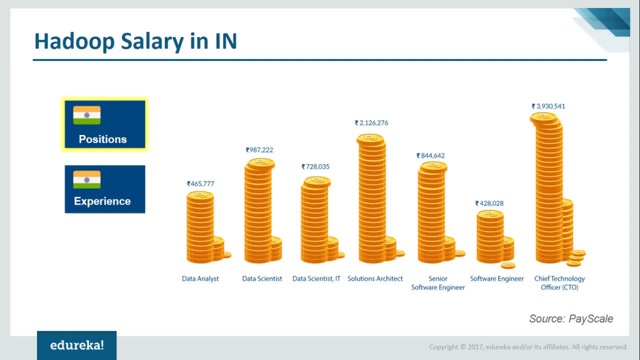 in India. So the different positions in India as a big data professionals are data analyst, data scientist, data scientist in IT solutions architect, senior software engineer, software engineer and chief technology officer or CTO. So as a data analyst, you might expect. your salary to range somewhat from 4.6 lakhs, But as a CTO, you'll be starting with 39 lakhs. Now your salary will also vary according to your experience. So if you have less than one year of experience, you'll be starting with 4.3 lakhs. However, if you have more, 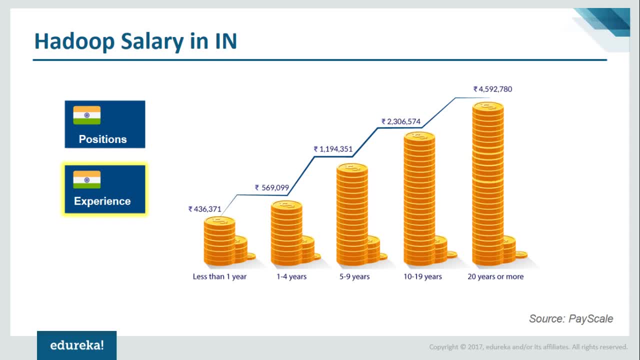 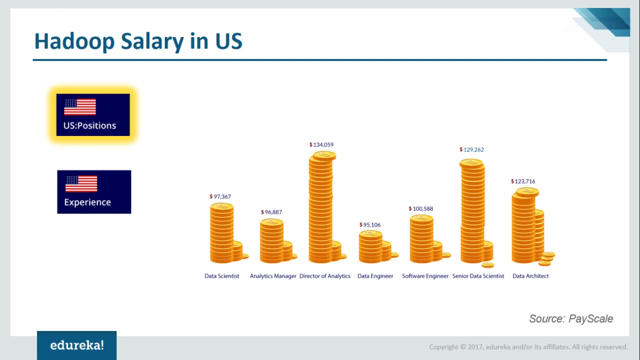 industry experience. you'll be starting with 45 lakhs, And here I'm talking about the general industry experience. All right, So your salary will vary according to positions and experience. And here are the salary trend of big data Hadoop professional in US. Again, I've categorized it according to different. 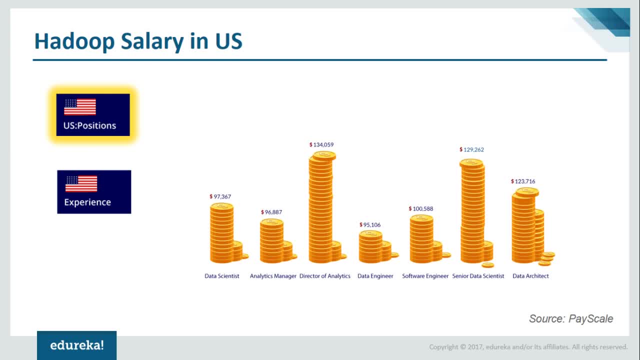 positions and experience. So the different positions of a big data professional in US are data scientist, analytics manager, director of analytics, data engineer, software engineer, senior data scientist and data architect. So as a data scientist, you'll be starting. 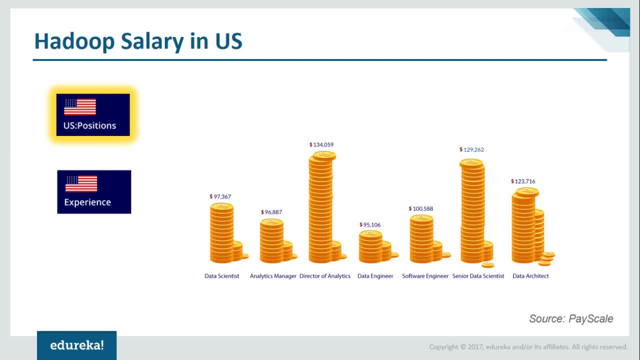 with $97,000.. And as a director of analytics US, you'll be starting with 4.3 lakhs. So if you have less than one year of experience, you will get around $135,000.. Again, it also 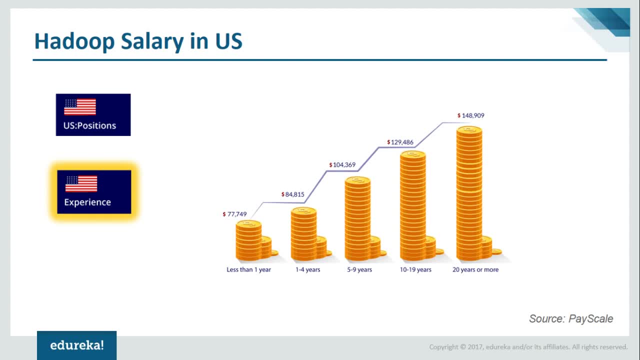 varies according to your experience. So if you have less than one year of experience, you'll be starting with $77,000. And if you compare it to the salary of that with the big data professionals in India, of course US is paying them a lot more, So maybe you. 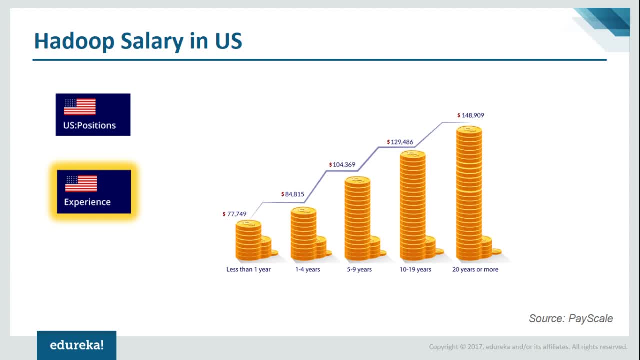 should all consider getting a job in US, right? All right, So let us move on and understand what is the market trend of big data and Hadoop, because obviously there are a lot of different things that are happening in the world. So 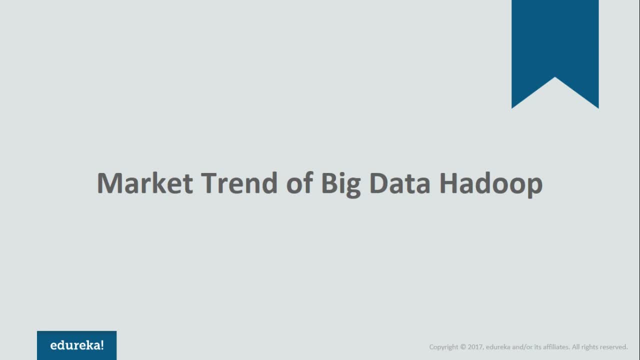 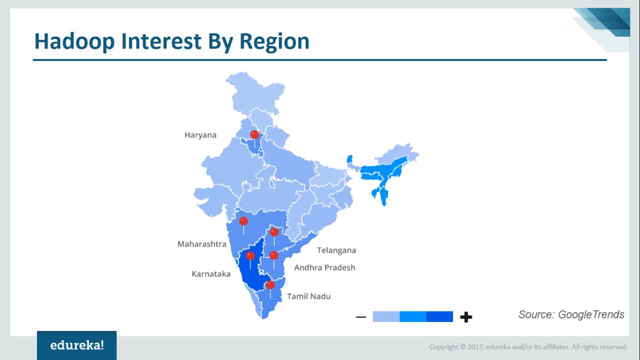 we are paying a lot to the big data professionals, But what will you do with all the salary experience if there aren't any jobs? But let me tell you that there are jobs and there are plenty. So I've listed down the top five states. in India, which has the maximum number of job? 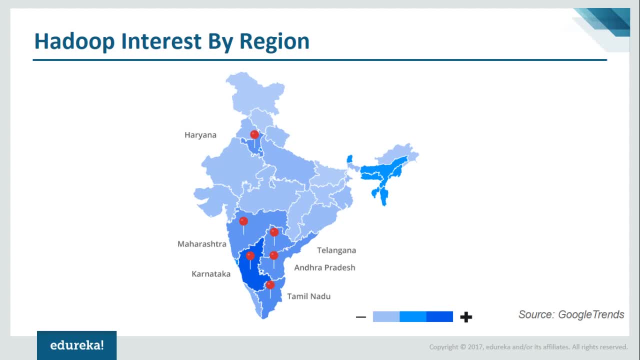 opportunities. So there is Karnataka in the darkest blue, And the darker the color of the state, it represents more job opportunities. So Karnataka is the darkest blue. It is because Karnataka has Bangalore, which is known to be the Silicon Valley of India, Apart from 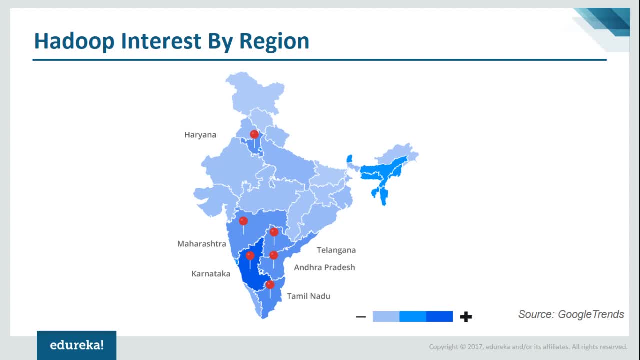 that there is Maharashtra, Telangana, Andhra Pradesh, Tamil Nadu and Haryana, And I think a lot of people might be surprised to see Northeast in dark blue, And let me tell you that of course, Northeast is not known for its tech, But whatever companies that are, 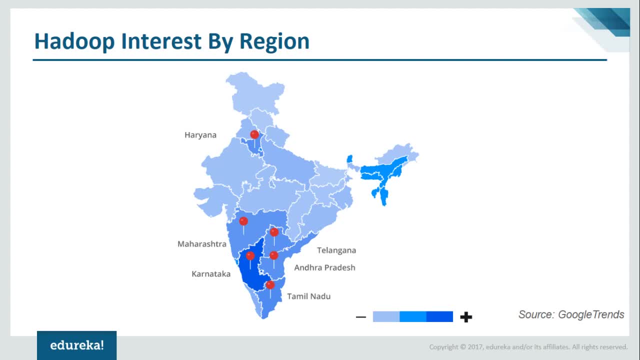 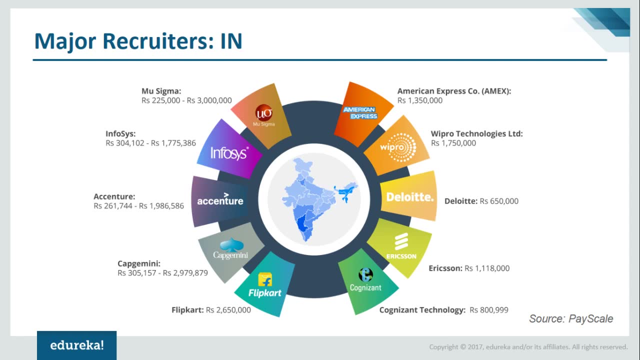 emerging in Northeast India are basically based on big data and Hadoop, And these are the major recruiters in India who are hiring big data professionals. I have also listed down the salaries they are giving out to the big data professionals. However, it will also vary according to the different positions and experience. So the top recruiters 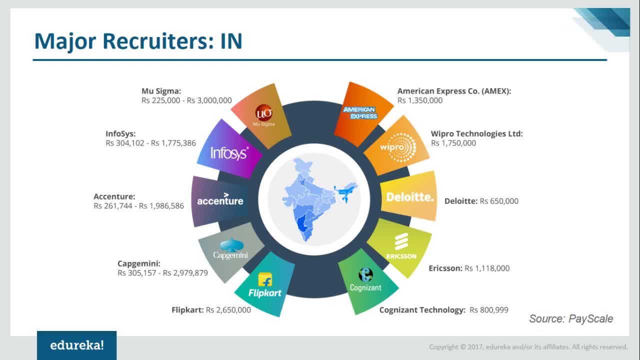 in India are Mu, Sigma, American Express, Wipper Technologies, Infosys, Accenture, Cape Gemini, Flipkart, Cognizant, Ericsson and Deloitte. However, these are just the top 10 companies, the big known names, But there are many other companies who are hiring big data professionals. 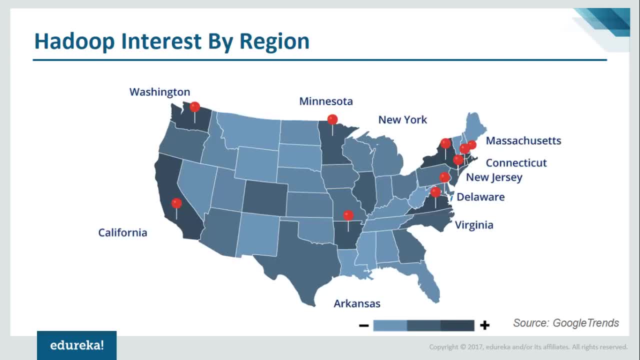 big and small in India, And here is Hadoop interest by region in the US. So here I have listed down the top 10 states with the most number of job opportunities similar to that of India. All right, So the top 10 states in US are Washington, California, Minnesota. 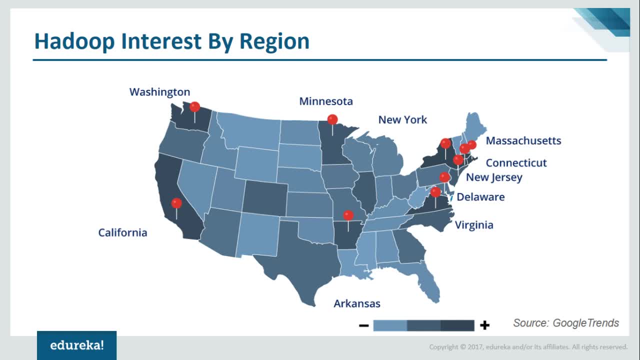 New York, Arkansas, Virginia, Massachusetts. I hope I pronounced that correctly. I always have a hard time saying that. Then there is Connecticut, New Jersey, Delaware. So again, there are jobs in other states as well. But I have just listed down the top 10 and I have 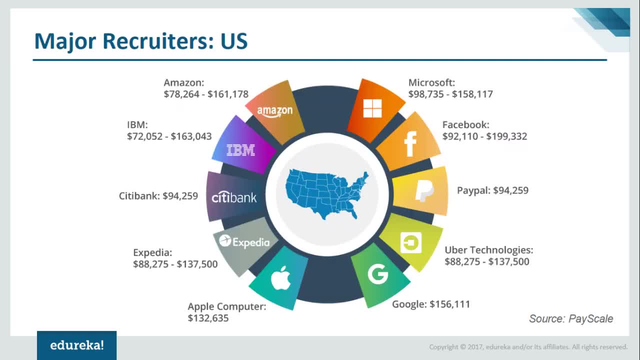 collected this from Google Trends. And these are the major recruiters in US, the big names that you already know: Amazon, Microsoft, IBM, Facebook, Citibank, PayPal, Uber Technologies, Google, Apple Computer and Expedia. And again, I will tell you the same thing: that there are lots of other companies. 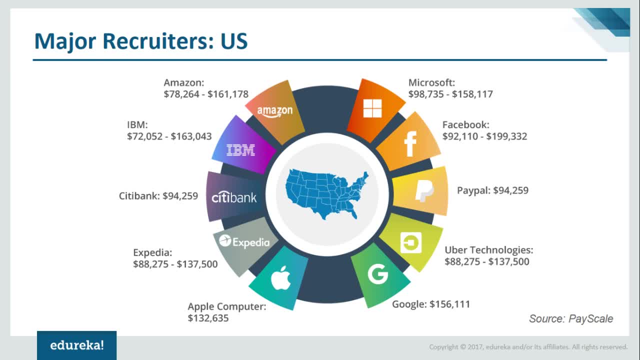 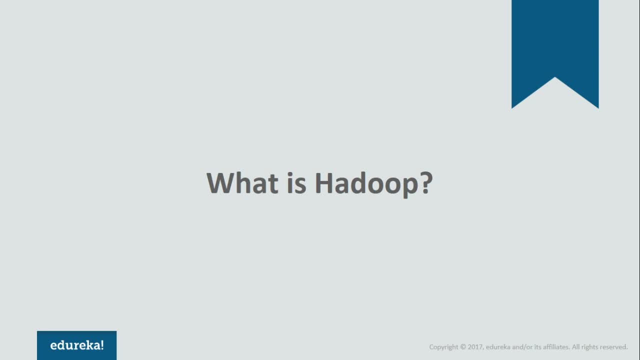 who are hiring big data professionals in US as well. So I have talked about the salary you can expect as a big data professional and the market trend, just to show you that there are a lot of jobs available for big data professionals. And let me also tell you a very interesting fact that I have just read in Gartner recently. 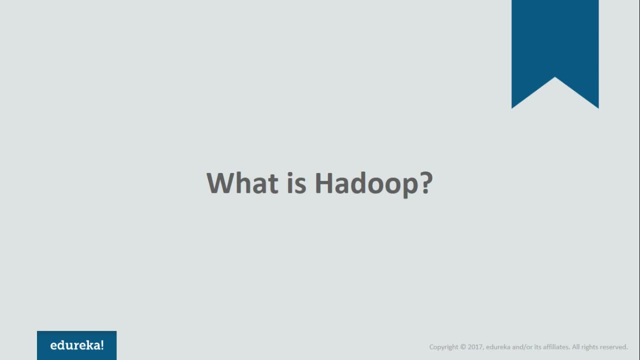 They have published that by the end of 2019, there is going to be a scarcity of big data professionals and the scarcity would go up to 190,000 big data professional in just US. So it is going to open up a lot of opportunities in India and the South Pacific area as well. 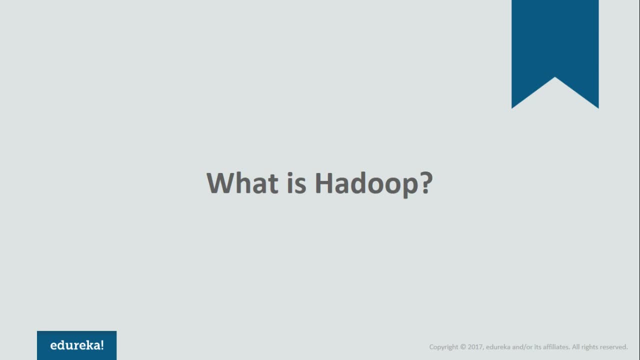 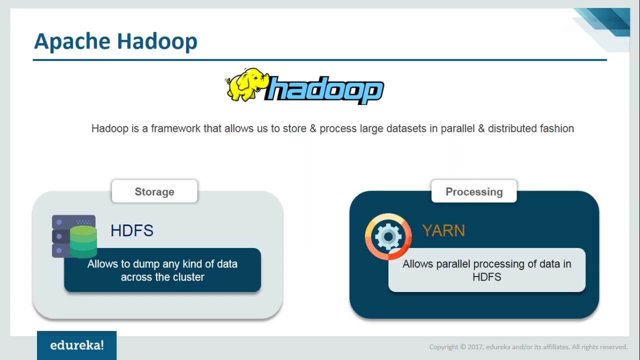 Okay, So we have done with the salary trade, We have done with the market trend and the market trends. So let us try to understand what is Hadoop. So we will go through some fundamentals of Hadoop now. So let us see what is Hadoop. So Hadoop is a framework that allows us to store and process. 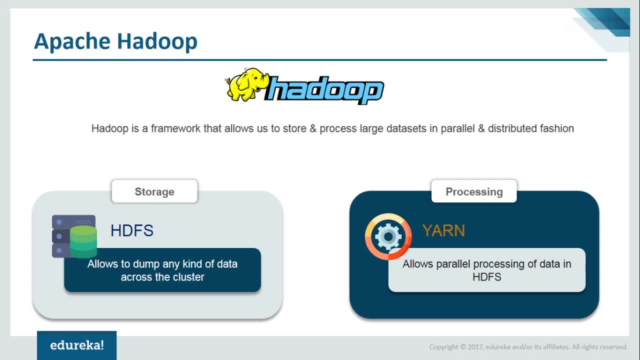 large data sets in parallel and distributed fashion. So what was the main problem? that was related to big data. So the first problem was to store all the data, And that is why Hadoop came up with a distributed framework to store data, which is known as HDFS, And it allows to dump any 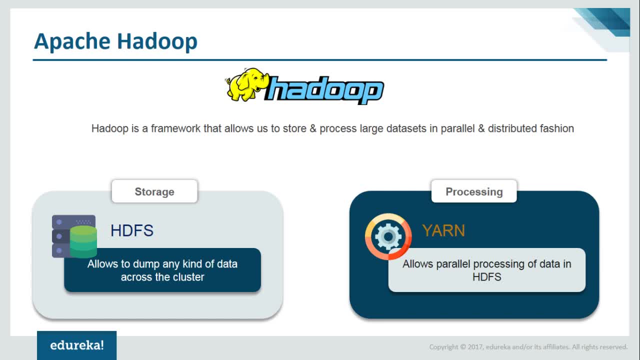 kind of data across the cluster. Let it be structured data, semi-structured data or unstructured data. You can dump anything in HDFS, And the next problem related to big data was to process it, And hence Hadoop came up with YARN. YARN stands for Yet Another Resource Negotiator, And this allows parallel processing. 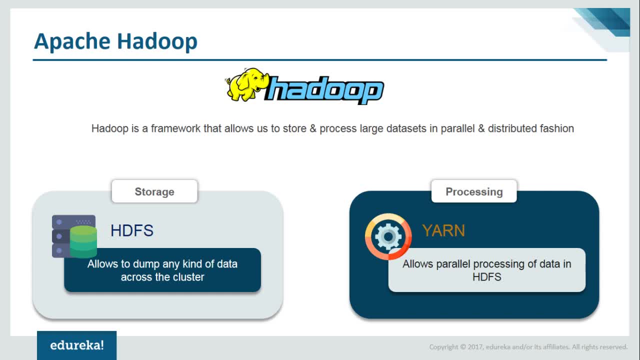 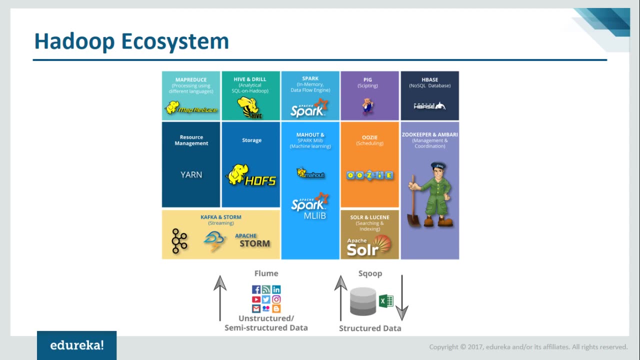 of data that is stored, distributed in HDFS. So this is how Hadoop has solved the big data problem. So by storage HDFS and processing with YARN. And the best part about Hadoop is that it can integrate a lot of different tools together. 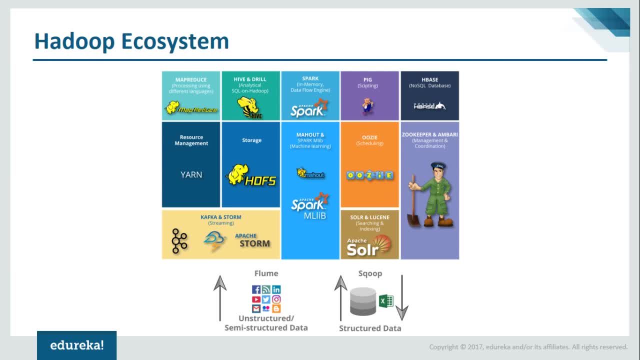 And it makes up the entire Hadoop ecosystem. So let me tell you, give me so just. I'll just give you a brief introduction to all these different tools. So there is MapReduce. So this is the core component of processing in Hadoop ecosystem because it provides the 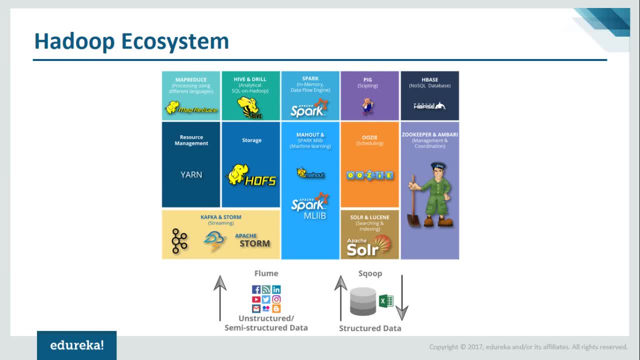 logic of processing. So it is basically a software framework that helps in writing applications in different programming languages. Like you can use Java, Scala, etc. Then I've already talked about YARN and HDFS And, don't worry, I'll be telling you more. 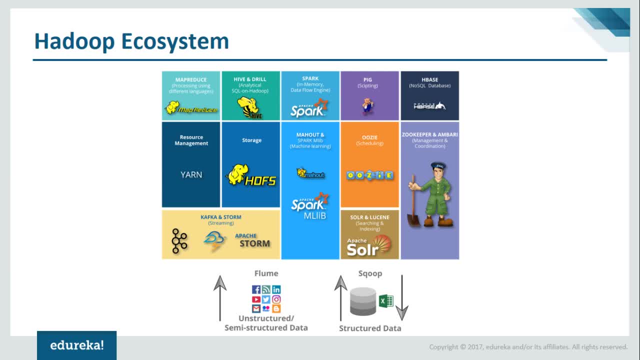 about HDFS and YARN in the coming slides. Then there is Hive, which is a very popular analytical tool. So this was developed by Facebook. It is because they have been accumulating a lot of data and they wanted a SQL like query language in order to analyze that data. 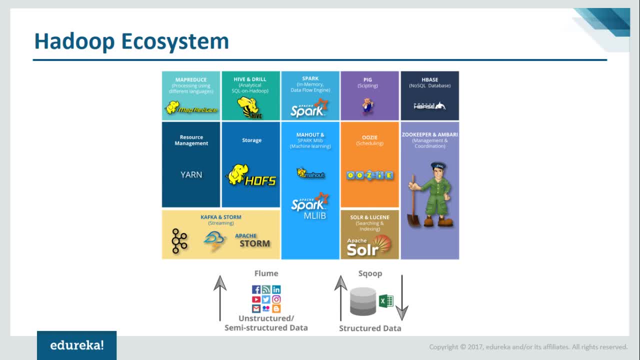 And hence they came up with Hive query language. So, and hence Hive. And then they have donated Hive to the Apache Foundation And it became a part of the Hadoop ecosystem. Then there is Apache Spark. I'm very sure that if you have ever Googled about processing big data, you have come across. 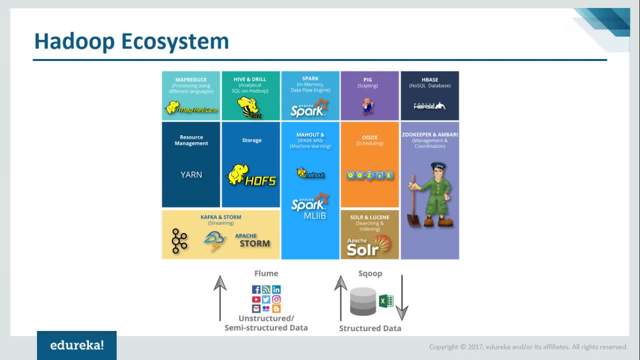 Apache Spark. It is a very popular tool in order to process real time data. Then for scripting you have got Pig, which is again created by Yahoo, And then they have made it open source and donated it to Apache Foundation. Then a NoSQL database, which is EdgeBase. 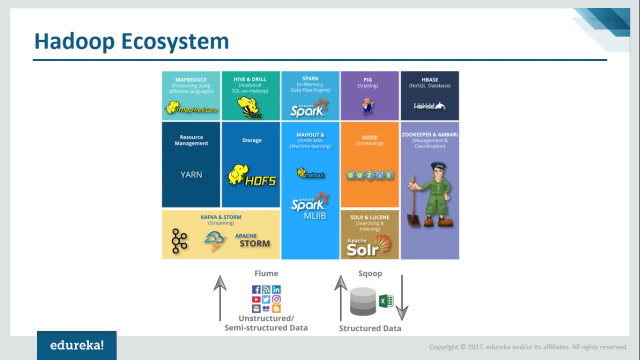 Then you have got different machine learning libraries, Things like Mahoot and Spark MLLib. So these are libraries that contains different machine learning algorithms on which you can train your model on. Then for scheduling you have got Uzi. For searching and indexing you can use Apache, Solar and Lucent. 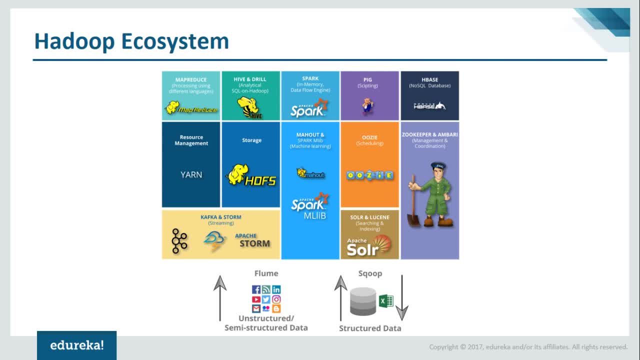 Then Kafka and Apache Storm. Now Apache Storm is highly optimized to process real time streaming data And, in order to streamline all the processes together, you can use Apache Kafka And then you can use Zookeeper and Ambari, because you can use all of these tools together, or 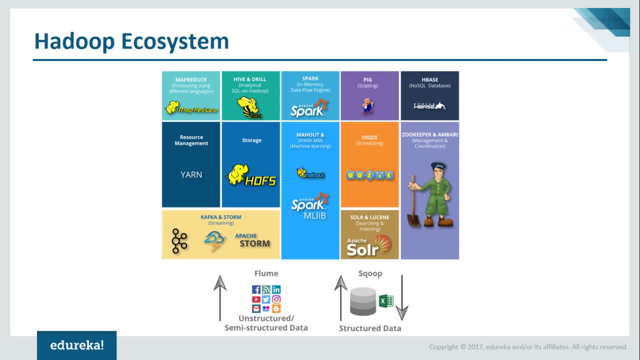 you can use. We might be using few of these tools together, right? So if you want to orchestrate this process of managing all the tools, you can use Zookeeper and Ambari for management and coordination, And in order to ingest the data into HDFS, you can use different tools like Flume or 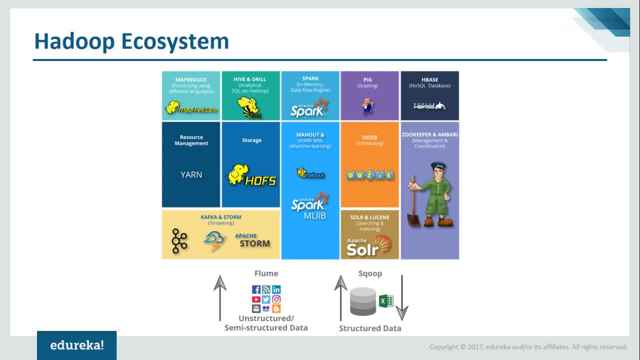 Scoop. So Scoop is used to ingest only structured data into HDFS, and Flume is used to ingest unstructured and semi-structured data. So I'll be telling you more about Flume and Hive, because that is what we're going to use. 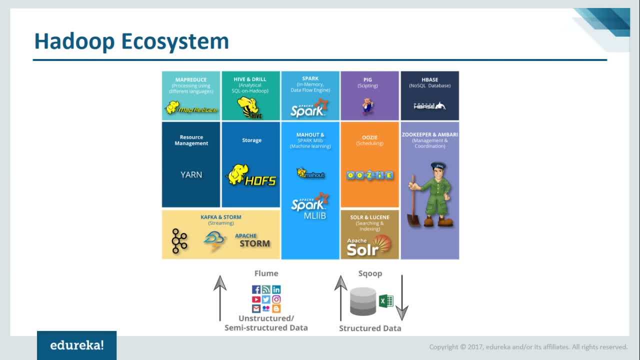 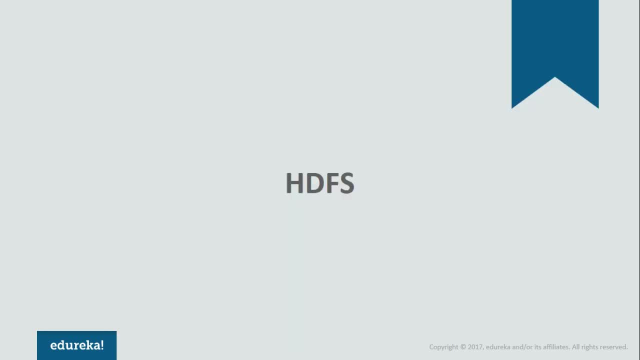 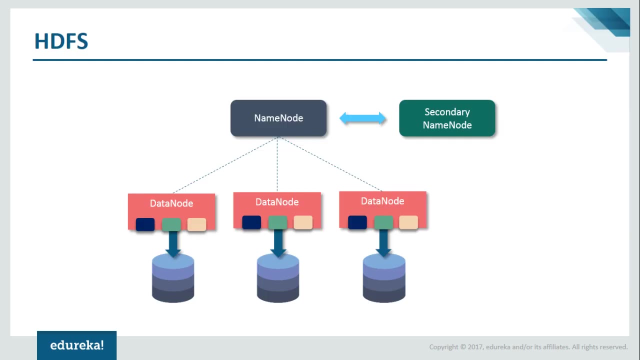 in our Twitter analysis. Alright, so I hope that you have got an overall idea of all these different tools in the Hadoop ecosystem, Alright, so now let us move on to HDFS, which is the storage component of Hadoop. So these are the daemons that run on HDFS. 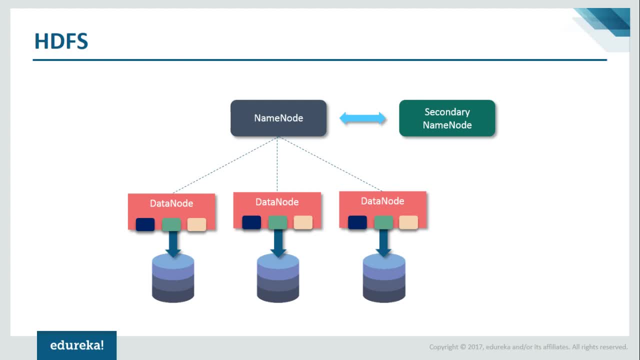 Daemons are nothing but processes. So this is laid out in a master-slave topology: The master daemon is known as the name node and the slave daemon is known as the data node. So data node is actually the place where you're at. 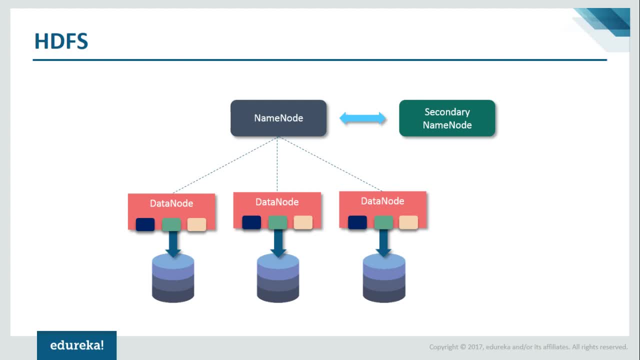 Actual data is stored into different blocks and the name node manages all the data nodes. And how does it manage all the data nodes? So basically, the name node keeps a metadata of what data is contained in which data node. So basically it manages a sheet. that, okay, this data node has this data block data node. 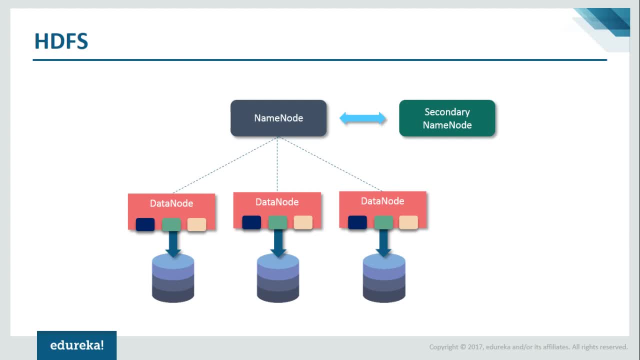 two has data block number four, something like that. So it manages the metadata to keep a track of what data is contained in which data node. And if you're thinking that, Okay, There is one more box that you can see which is called secondary name node. 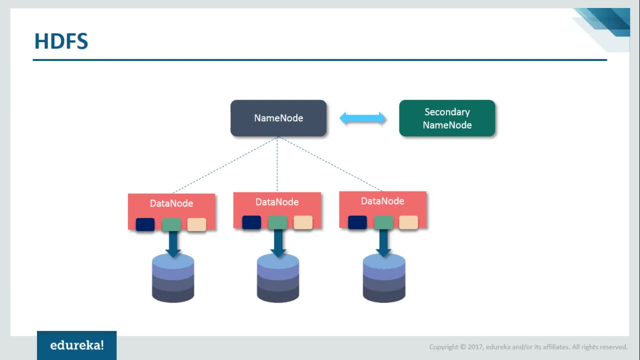 So this is also a daemon, But if you're wondering that, whether it is a backup name node, no, So secondary name node is basically an assistant to name node, Since I told you that the name node manages a metadata, of which data is contained in which? 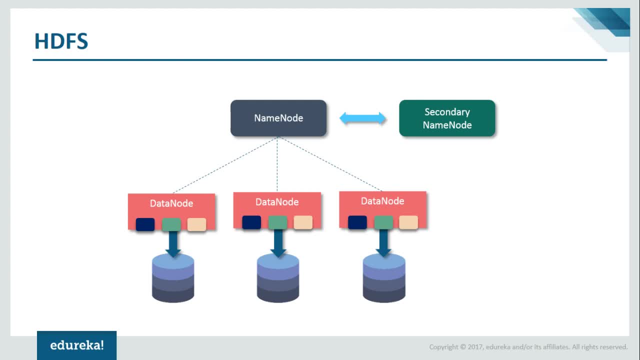 data node, the secondary name node, helps the name node or assist the name node in managing that metadata. All right, And like how you report to your managers, The same with data node also reports to the name node in the form of signals, which are: 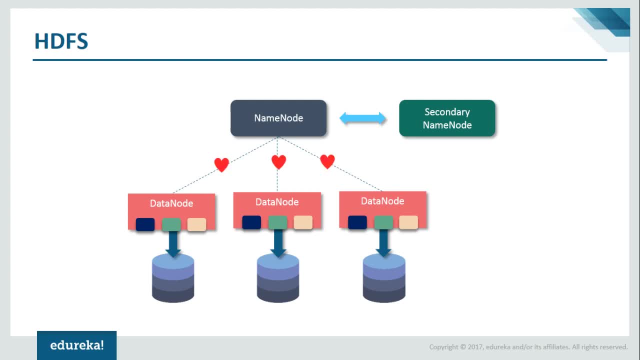 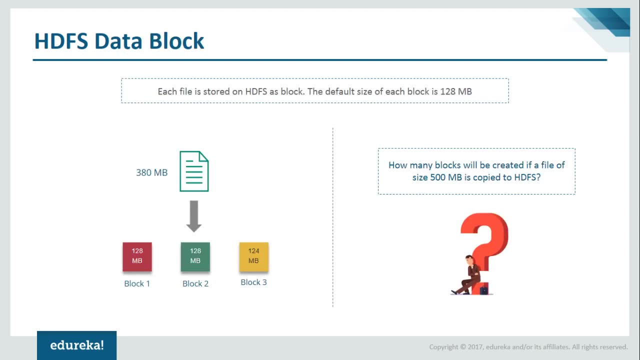 known as heartbeats. So this heartbeats are just to inform the name node that this data node is alive and is functioning properly, All right. And since I have told you that in HDFS your data is stored in different blocks, 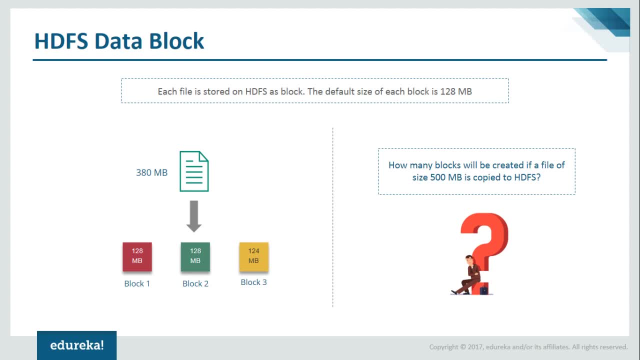 So the default size of each of the block is 128 MB. So let's say that if you have a file of 380 MB, Okay, It will be split it up into different blocks of 120 MB each. So with a file of 380 MB, the first block will occupy 128 MB. 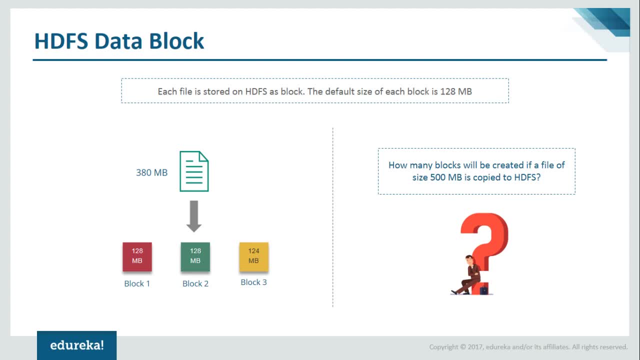 The second block will occupy 128 MB and the third block is occupying just the remaining memory, which is 124 MB. So I have a question for you guys. I would love if you try it out. So let's say that you have a file of 500 MB. 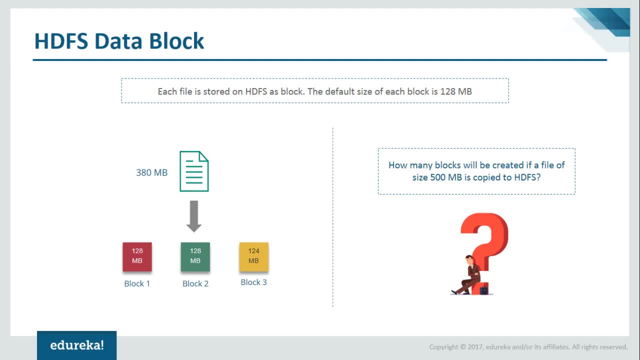 So how many blocks will be created? Come on, It's a very easy one. I would like, if you, just give me some answers. All right, You can leave your answers on the chat box and if someone have answered four, congratulations to everyone who have answered four blocks. you are absolutely correct. 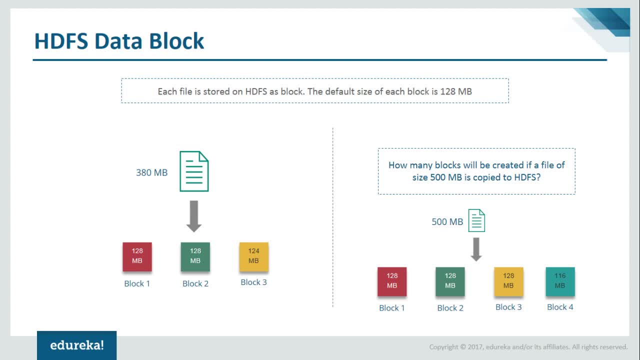 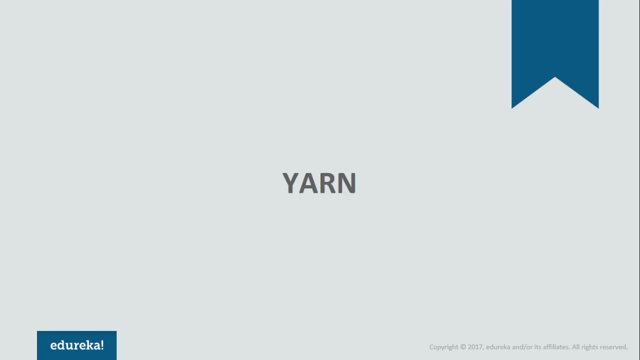 So the first three will occupy 128 MB and the last one will just occupy 116 MB. All right, So I hope that you have understood how data is stored in different blocks in HDFS. So now let us move on and understand about the processing unit of Hadoop, which is YARN. 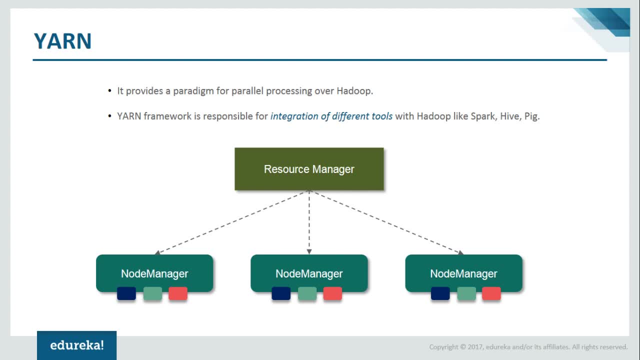 Now, since I've told you that Hadoop can integrate a lot of different tools together, so YARN is solely responsible for the integration of different tools together with the Hadoop framework. All right, And here are the daemons that run on YARN. 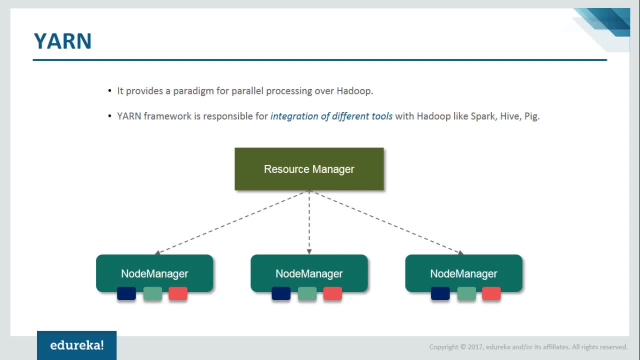 Again, this is a master-slave topology. The master daemon is known as the resource manager and the slave daemons are known as the node managers. And node manager is actually the daemon, is actually the place where the actual processing happens. Okay, 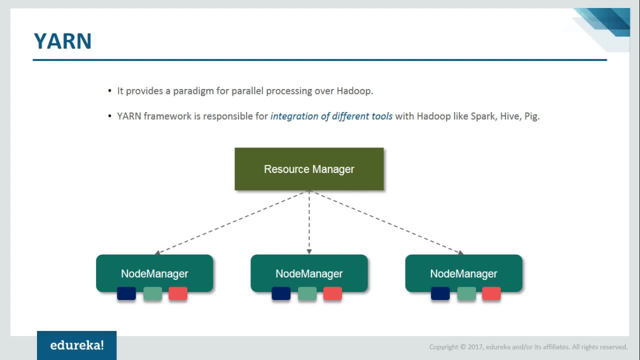 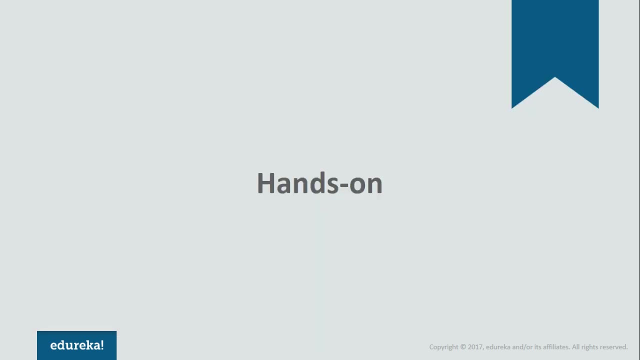 This is where all the data blocks that are stored in HDFS gets processed in the node manager And the resource manager just manages the node managers by providing all the resources that is needed in order to run a particular job in the node manager. So this is how HDFS and YARN works. 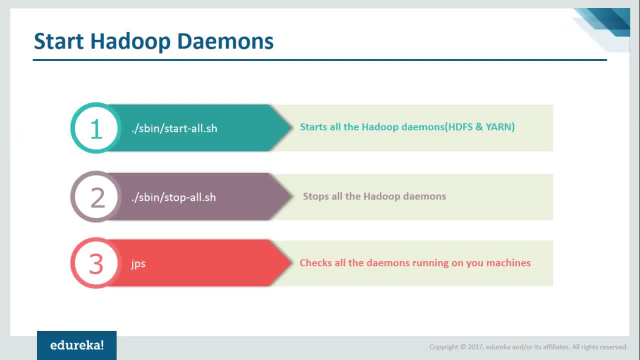 So here are some basic commands that you can try on. Okay, So if you want to start all the HDFS and YARN daemons, you can use this command. Make sure that you go to the Hadoop directory and run this command: /sbin/startallsh. 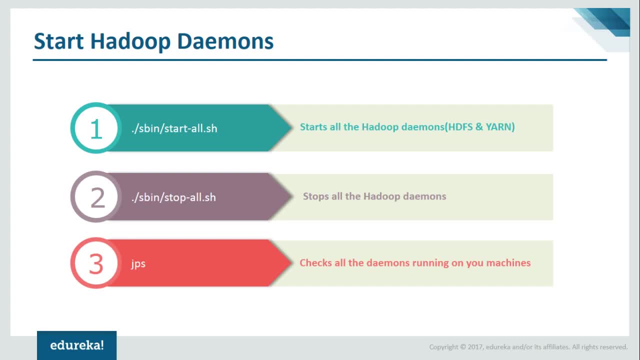 So it will start all the HDFS and YARN daemons, like your name, node, your secondary name, node, data node, resource manager and node manager. And if you want to stop all these daemons, use the same command, only replace, start with. 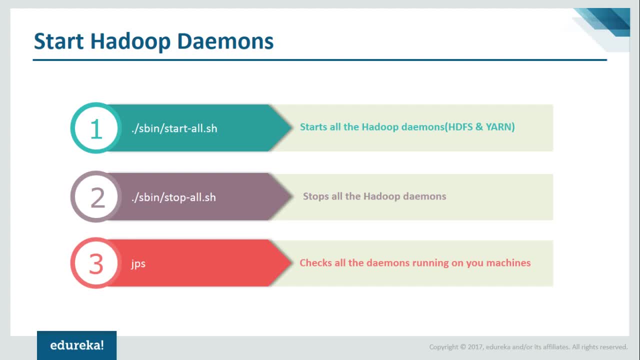 stop, And if you want to check if all the daemons are running, you can use this command: JPS. So I'll be showing you during the hands-on part where I'll be doing the Twitter analysis. All right, So now just let us move on and give you a brief description of what we're going to do. 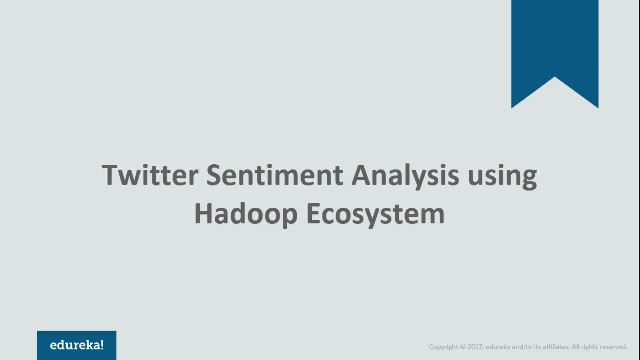 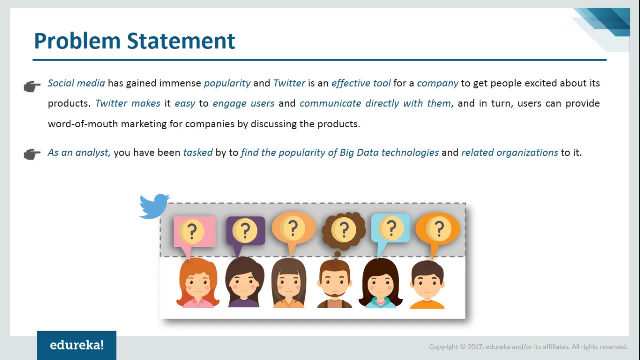 So we're going to do a Twitter sentiment analysis using the Hadoop ecosystem tools, All right, So we're going to find out that how popular big data and Hadoop is Okay, So, and what is the best way to find out about the popularity of something? 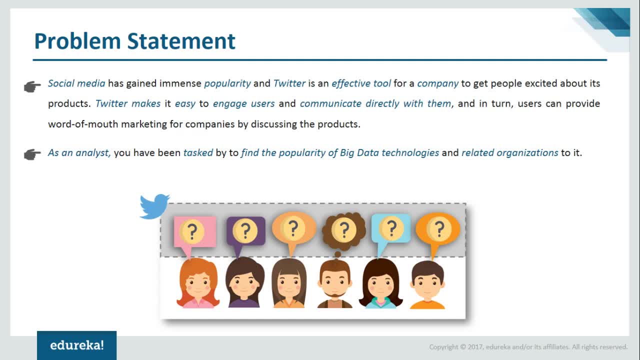 Of course, Twitter. If people are tweeting about some particular topic, definitely there is a fuss going on about it, Right? So we'll try to find out how much activity is going on in Twitter about big data and Hadoop. All right, 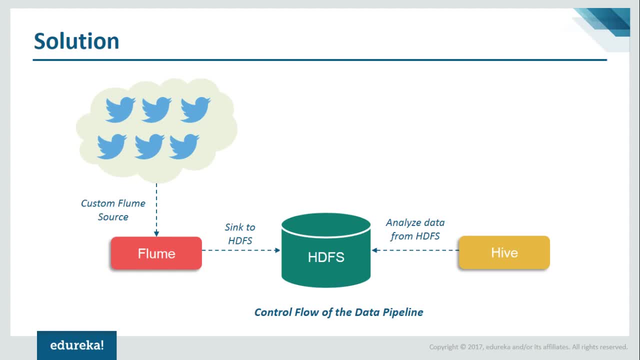 So let me just show you how we're going to perform. So I have laid out a solution strategy of what we're going to do and how we're going to analyze all the tweets. So we'll be using two tools, Flume and Hive, and we're going to dump all the tweets into 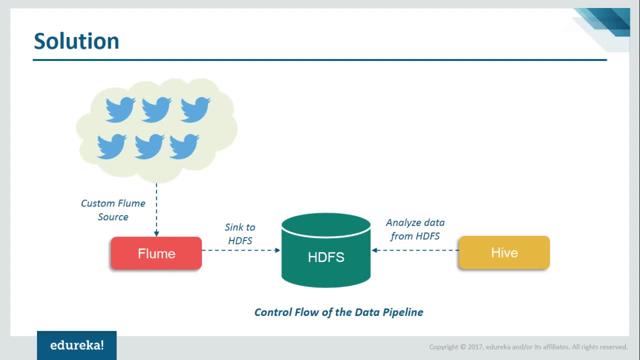 HDFS. So what we're going to do is that we'll fetch all the tweets and, using Flume, we'll ingest it into HDFS, And once all the tweets about big data and Hadoop are stored in HDFS, we'll analyze all. 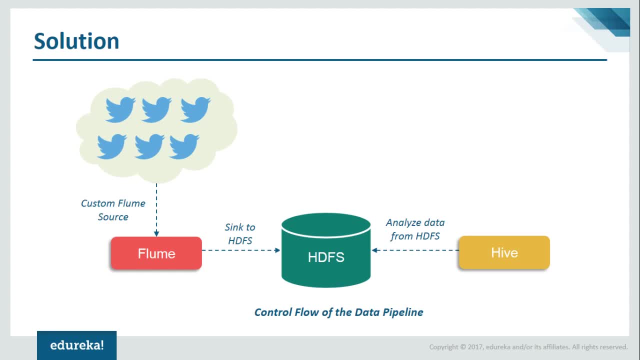 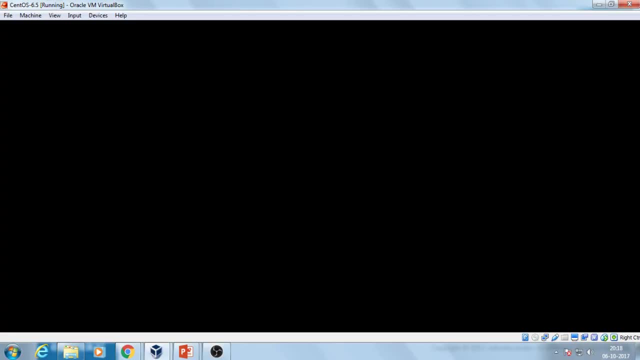 the tools using Hive. All right, So this is what we're going to do. So let me just go to my virtual machine, where I have set up on my Hadoop cluster, All right, So I hope that you're able to see my screen. 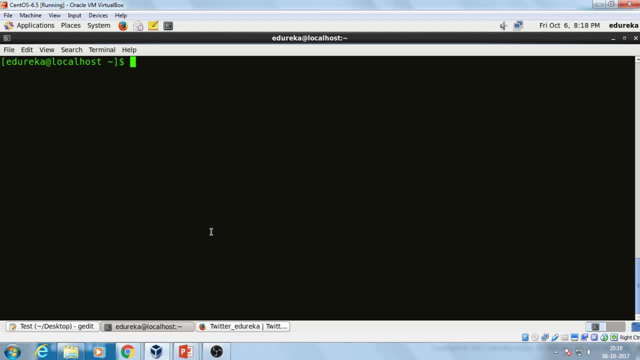 I want some confirmation That you're able to hear me properly and also see my screen All right. So I guess you're able to hear me and see my screen right, Okay? So let me just show you what are the daemons running here. 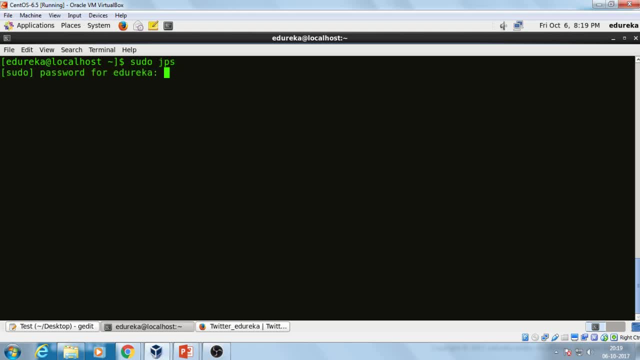 So I'll just run this sudo jps. So it is asking for a password. Okay, So I have the daemons that are running in my virtual machine. This is all the daemons, the HDFS daemons. data node. name node: secondary name node. 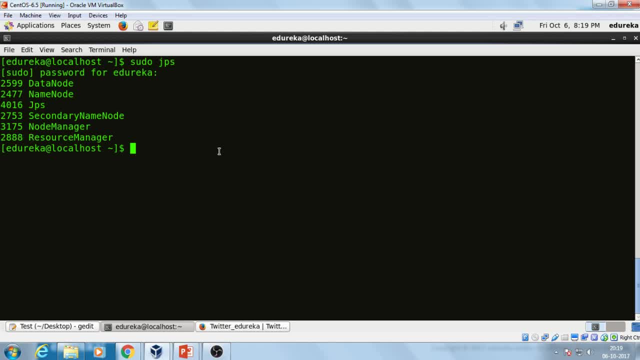 and the yarn daemons: node manager and resource manager. All right, So now let me show you how to do the Twitter analysis. So first thing we need to do is that we need to run a Flume configuration file. Okay, So let me just show you where that file is. 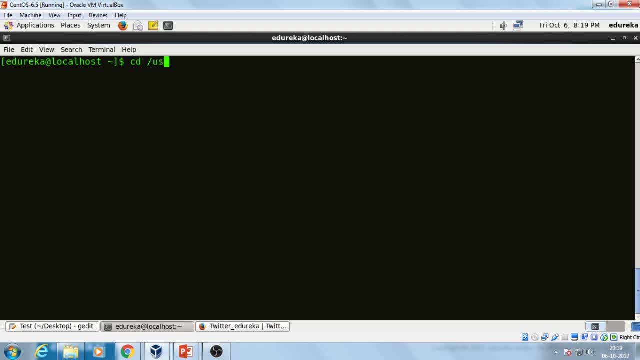 So I'll be just moving to the directory which contains my Flume configuration file That I need to run in order to fetch all my tweets. So it is in user lib. then there is flume-ng and I have to go to the bin file which contains. 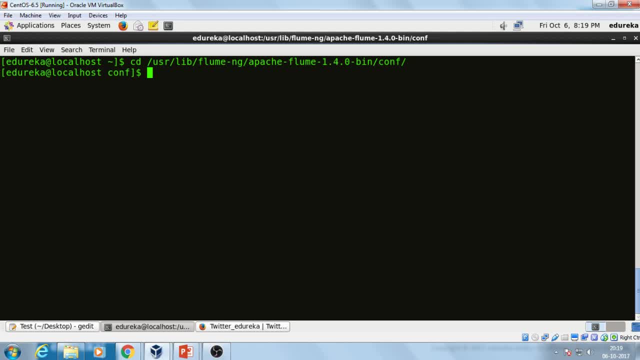 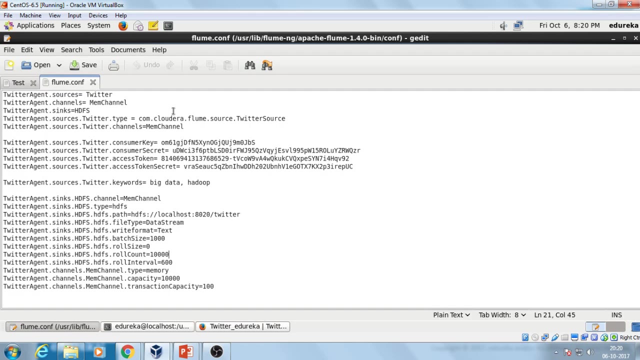 my configuration directory. All right, So here is my flumeconf. So let me just open up the configuration file and show you how it looks like. So I'll be using gedit. All right, So here is my flumeconf. 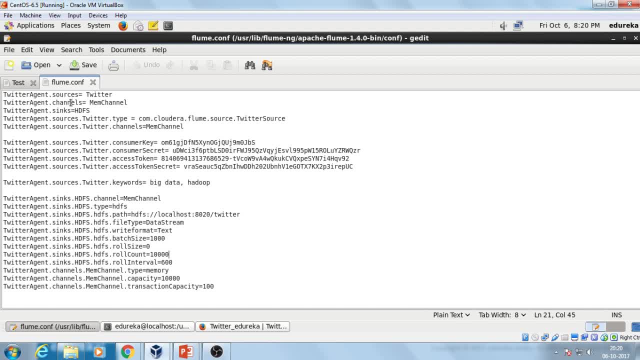 So we're using flume in order to ingest all the data into HDFS, and the data I'm talking about are tweets on big data and Hadoop. So in flume you've got three things. The first one is called source. 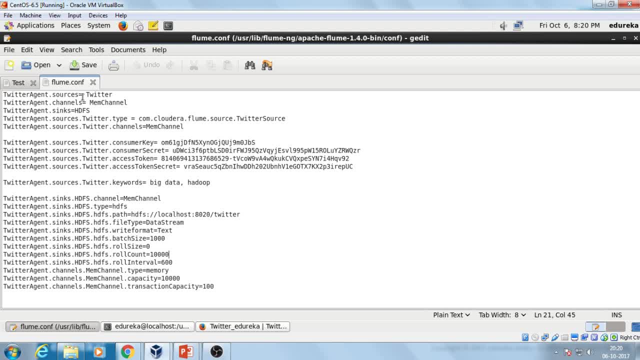 Now, source must be connected to the data source, and in this case, my data source is Twitter, because I'll be fetching tweets, right. And then the second thing is called sync. Sync should be connected to the destination where I'll be dumping all my data, or my tweets. 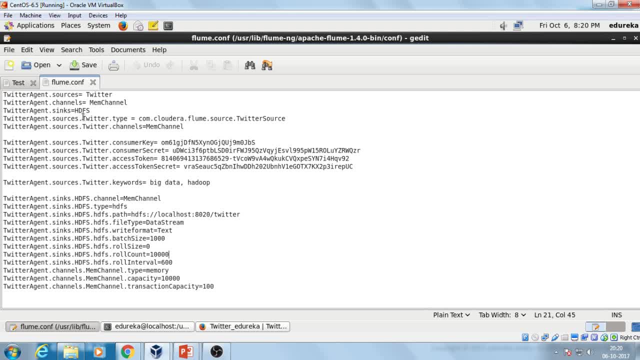 into, And in this case I'm dumping it all into my HDFS. so I've mentioned: sync is HDFS. And then the third thing is called channel. So channel is basically an intermediate buffer. So this is So a channel should be used. 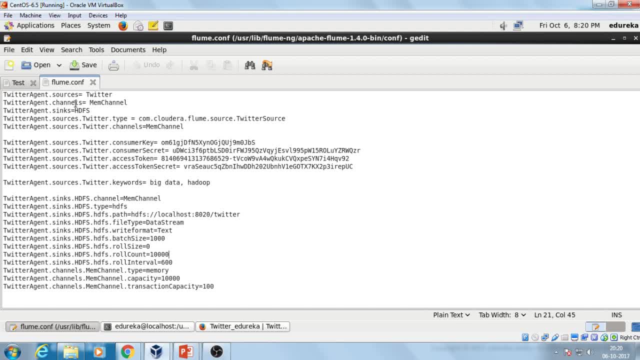 It is because you need an intermediate buffer, just because the writing and reading speed are different, right? You can also relate it to yourself, because obviously you can read faster than you can write with a pen on a paper, Right? So that's why I'm using a channel. 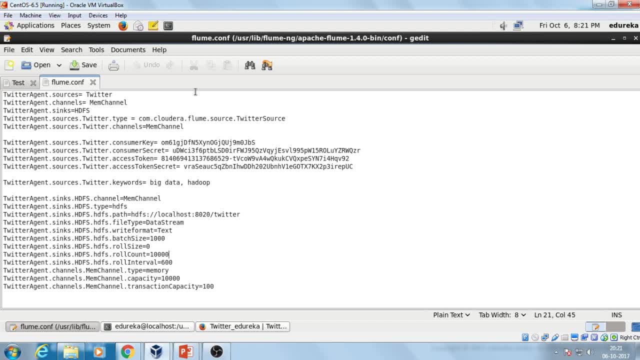 In this case I'm using my memory channel, So I've mentioned memchannel, okay, And then I want only the tweets, which has big data and Hadoop mentioned. So I've mentioned the keywords that I want: big data and Hadoop. 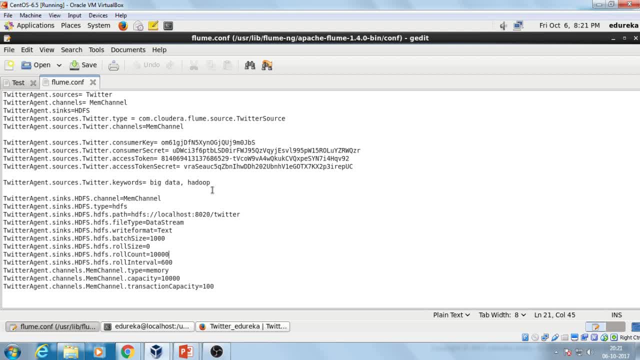 So it will get me all the tweets that has hashtag big data, hashtag Hadoop, or even the tweet has mention of this particular word: big data and Hadoop. So it will only fetch me those tweets And then, in order to connect to Twitter, 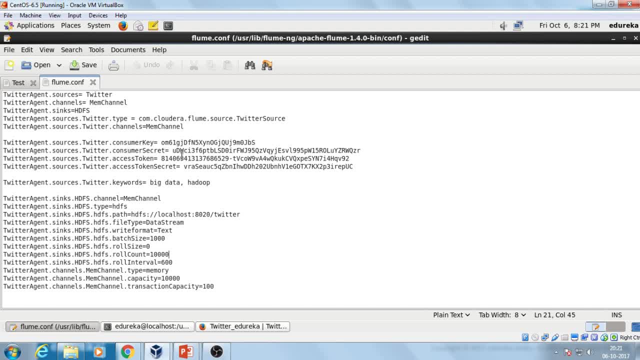 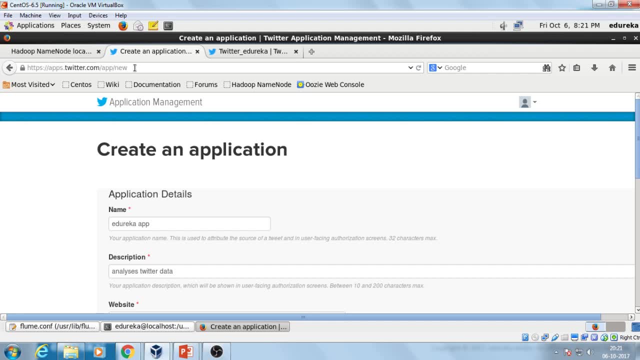 To connect to Twitter, you have to use certain API keys- consumer key, consumer secret key- And so let me show you where you can find this. So you just have to go to appstwitter. So here you can. There will be a button that says create new application, because, basically, whatever we're, 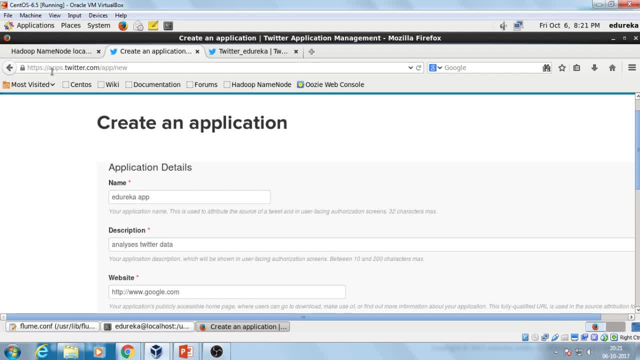 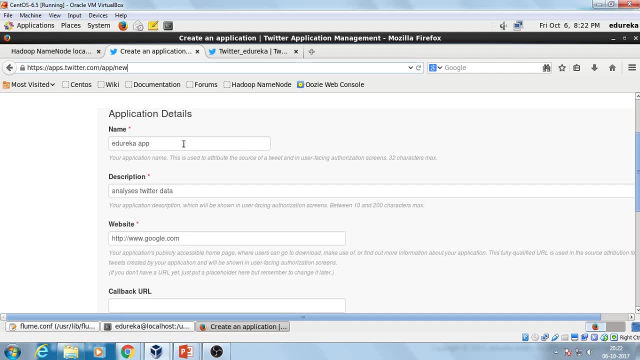 doing. we're creating a new application, So just go to this particular website, appstwitter. okay, So you'll find a form like this: So name your application And then provide a description, And also you'll find a form like this: 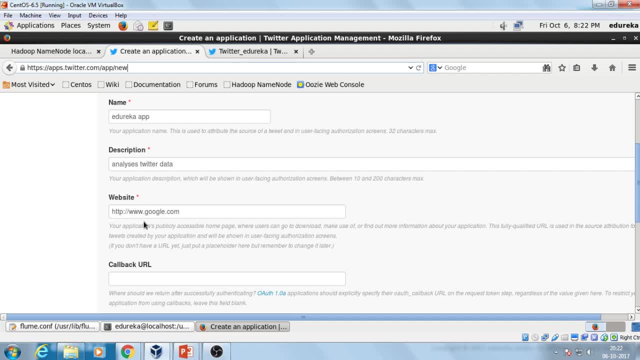 And also the website. So the website here basically means that the landing page of your application, And since we don't have any, you can provide it with any kind of placeholder, but make sure that you provide it in this format: http// and then the URL. 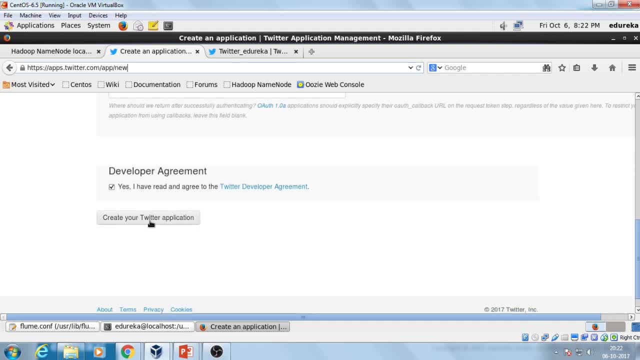 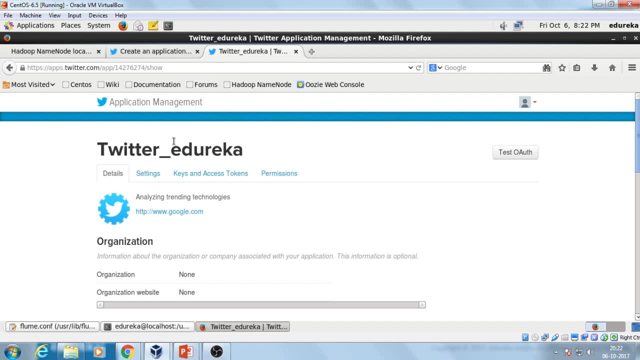 So basically, I've just provided googlecom- It is harmless- And then just take on this and create a Twitter application. Now I've already created it. So after we create your application, you're going to see something like this: So just go to keys and access tokens. 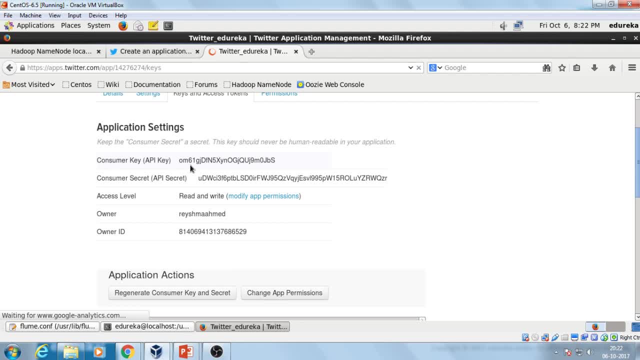 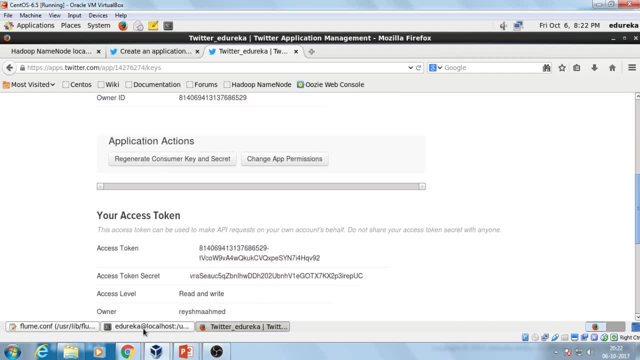 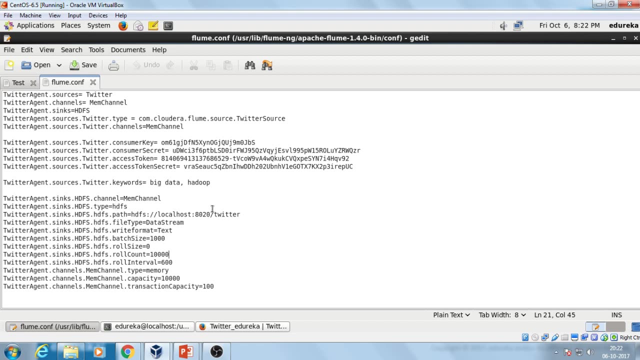 And this is where you'll be finding all your access tokens and your consumer API keys in order to connect to Twitter. So this is where I have copy pasted all the keys from in my configuration file. So let us go back. And I have also mentioned that. where would it get dumped in HDFS? 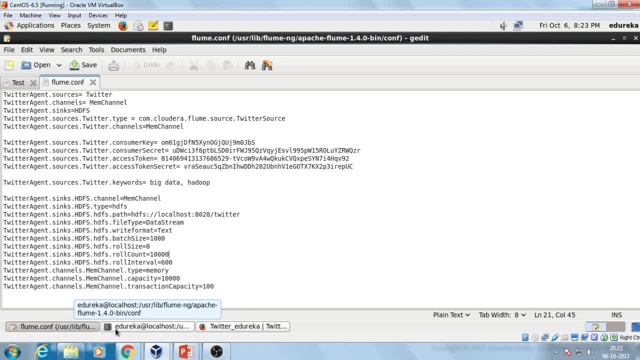 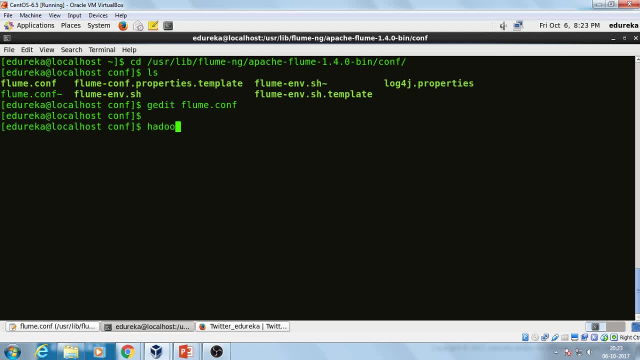 That will get dumped in a directory called Twitter. So let us go and create that directory. Okay, So For that creating a directory in HDFS, you have to use this command: hadoop, fs, make dir, And we're calling it Twitter. 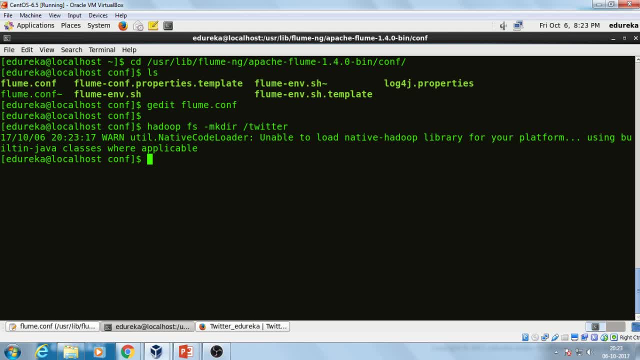 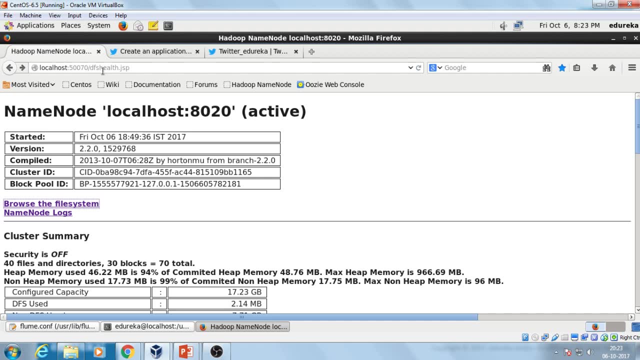 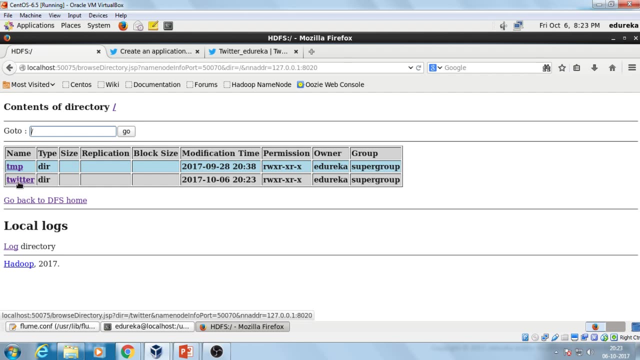 All right. So let me just show you the web UI for Hadoop, So you can just go to your local host, colon 50070.. So here you can just click on browse file system And you can see it has created the directory in my HDFS Twitter. 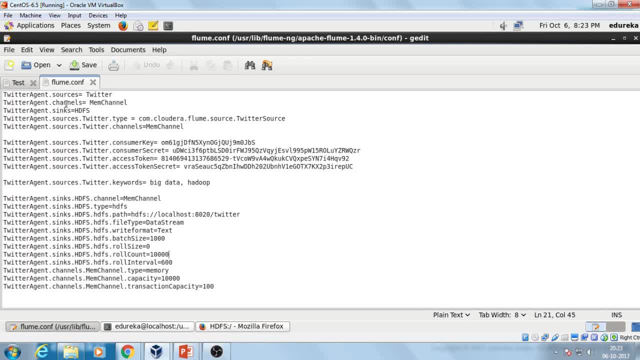 Okay, So let me just go to the flume configuration file. So this is my configuration file. I hope that you have understood what are the different components that I've mentioned here. So now all we need to do is run this particular file in order to fetch all the data from Twitter. 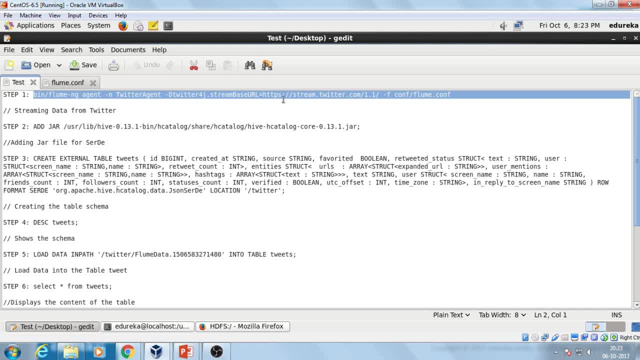 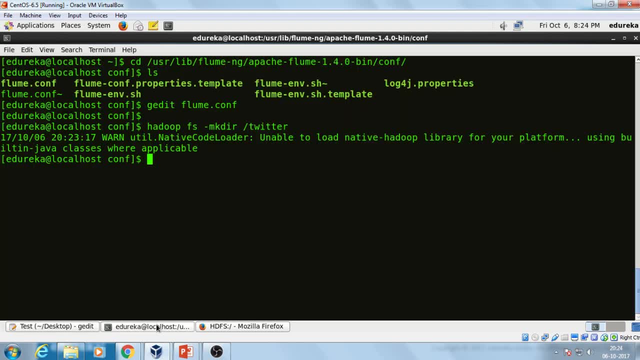 So for that you'll be using this command: bin flume, ng. You'll be running the configuration file in order to fetch all the tweets. Now I'm just pasting it only because I don't want any typos, because we don't have much time. 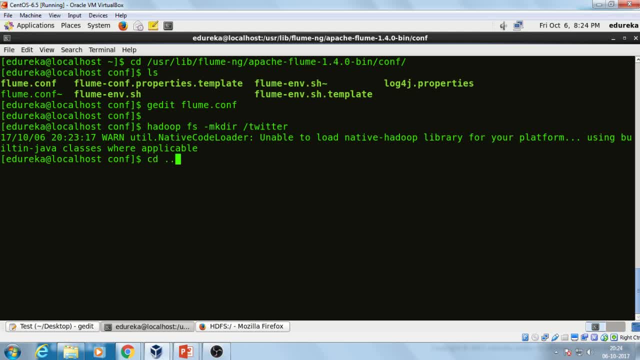 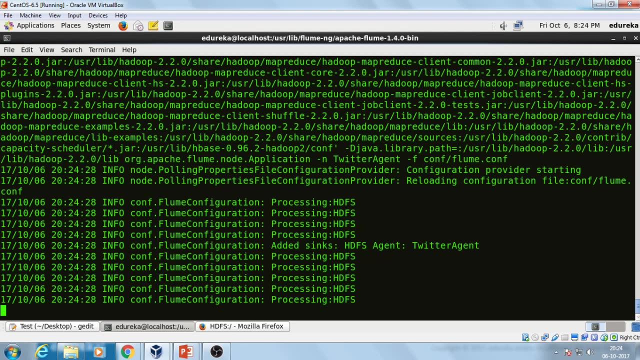 So for that you have to go to the folder, your bin folder, where you're. So this is my bin folder here I'll be running the command because I'm using my flume agent and it is in my bin folder, So I'll be just pasting it and enter. 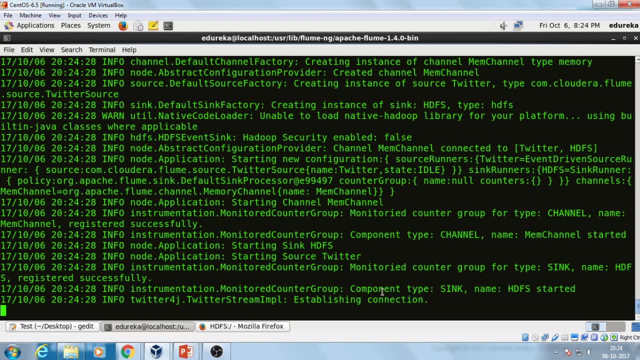 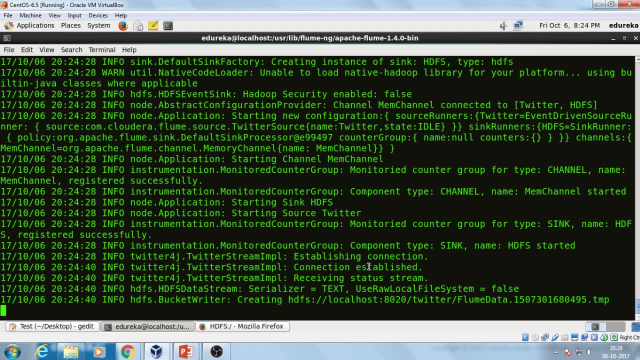 So this is going to fetch all the tweets related to big data and Hadoop, So it is establishing connection And the connection is established. So basically, now it is gathering all the tweets related to big data and Hadoop, So I'm just going to leave it on for a few seconds more, because we don't have much time. 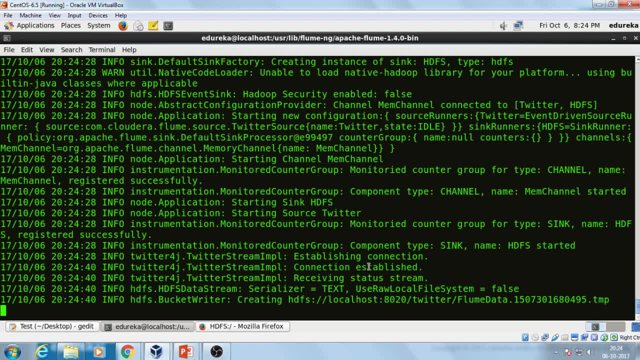 But when, if you try to perform this at your own home, you can just leave it for like half an hour, an hour so that you can fetch enough tweets about big data and Hadoop to get a better analysis of everything. Okay, So I'm just going to leave it for another few seconds. 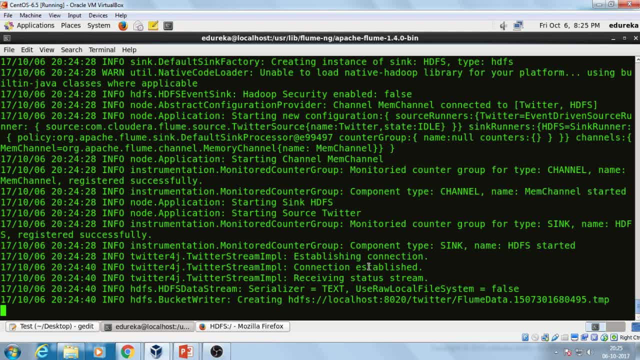 All right, So I guess five seconds more. So here you can see that in my HDFS, in my Twitter directory, there is one more file created. This is where all my tweets are getting stored. flume data, dot some numbers, dot TMP. 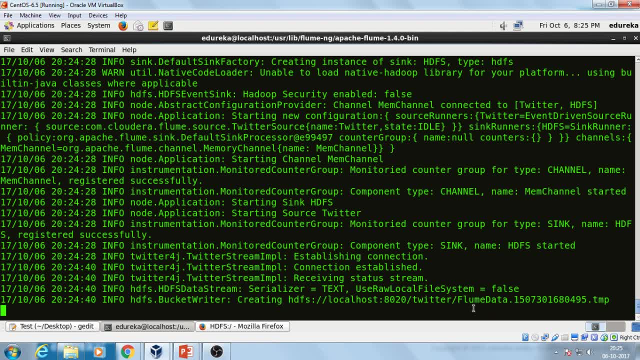 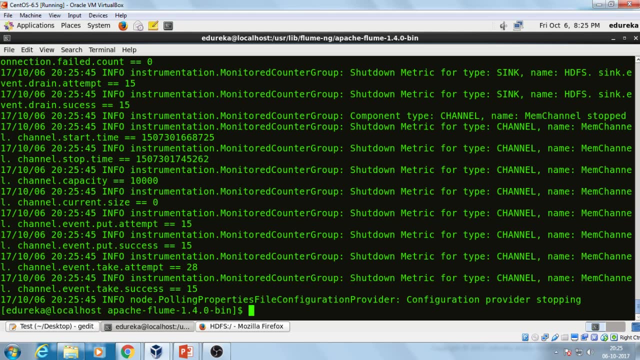 So this is another file that is created inside My Twitter directory, which is storing all the tweets. So I guess it is good enough to stop. All right, So I have stopped fetching tweets, So now let us go to my HDFS and check what data it has gathered. 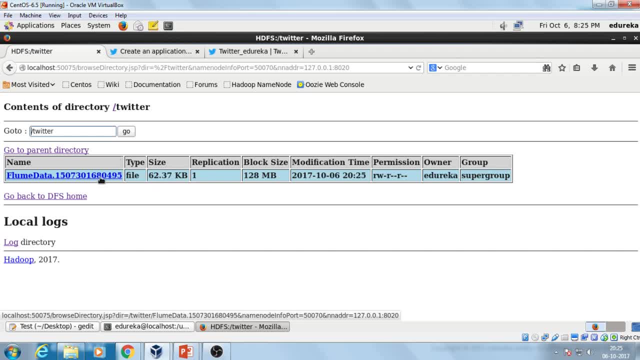 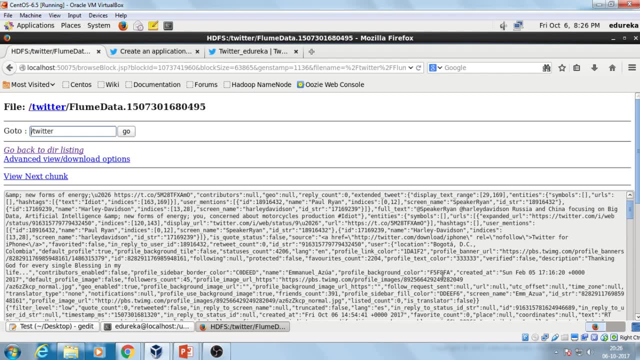 So it has gathered around 62.37 kbs of data. So if you click here, All right. So this are the different tweets, So this doesn't look very understated. This is understandable, because this is in a semi-structured format. 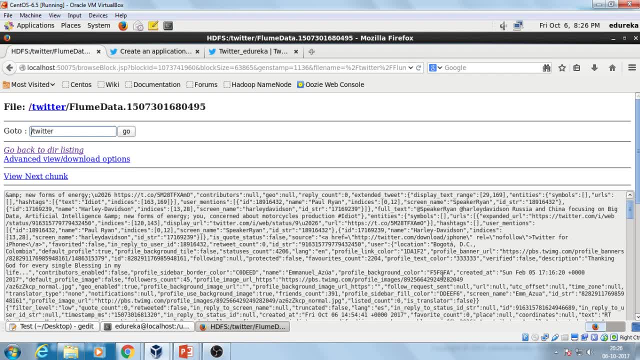 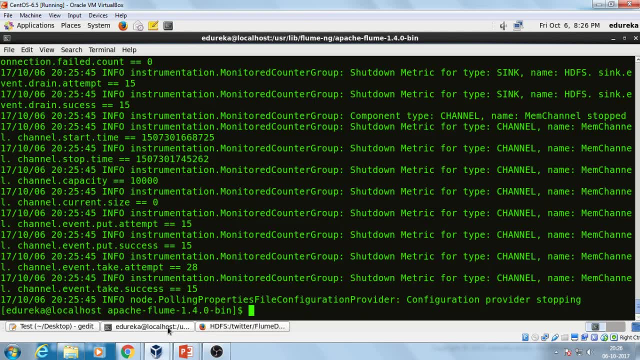 And, if you remember, I told you that flume is used to ingest unstructured and semi-structured data, And in this case we're dealing with a semi-structured data. Okay, So now I have fetched all my tweets. It is in my HDFS, right? 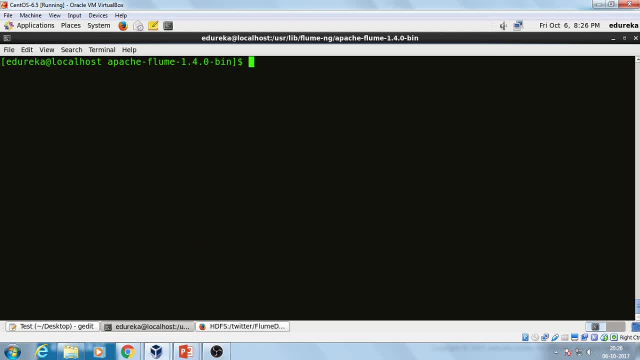 So all I need to do now is I need to analyze it, And for that I have to use Hive, And in order to go to my Hive shell, you just have to type Hive. Okay, All right, It is going to take a few seconds to get into the Hive shell. 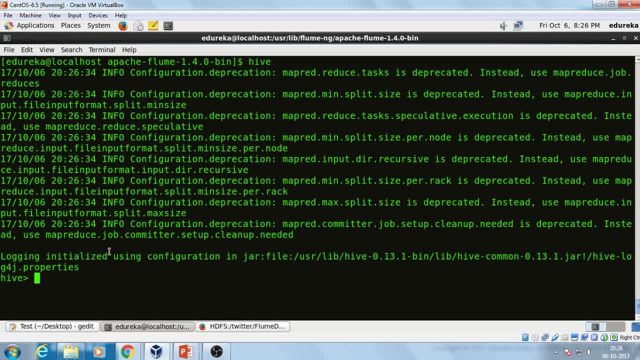 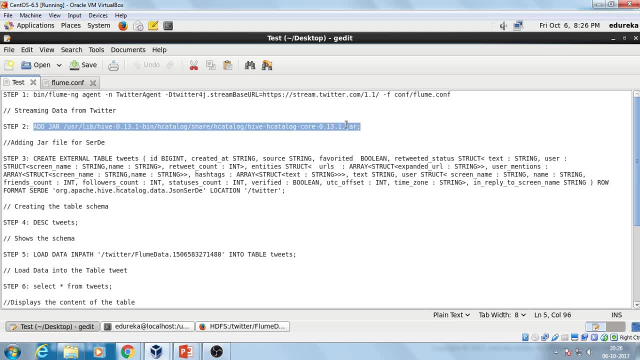 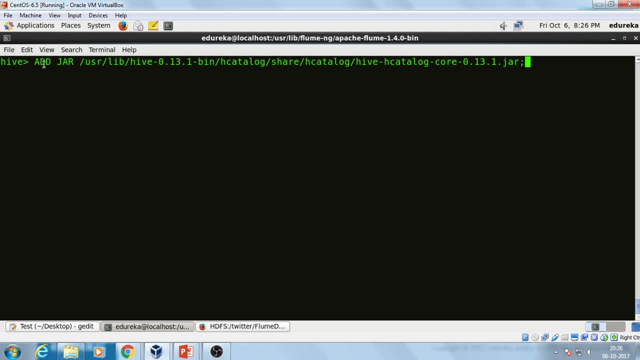 All right, So I'm in my Hive shell, So the first thing that I'm going to do is that I'm going to add a jar file. So this jar file is basically a surd. So this is the command in order to add the jar file. 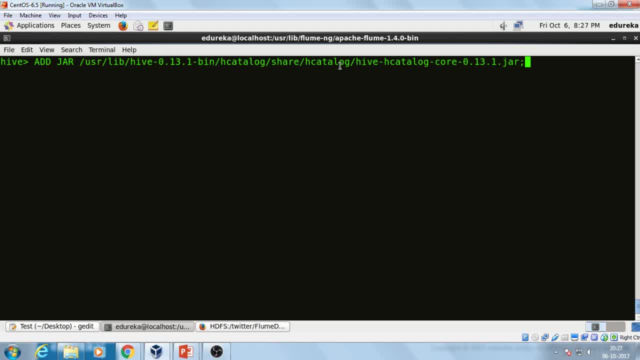 So add jar And I've mentioned the path in my file system where the jar file is located. Okay, So this jar file is actually a surd, and a surd is nothing but an interface that allows you to instruct Hive as to how a record or how a data should be processed. 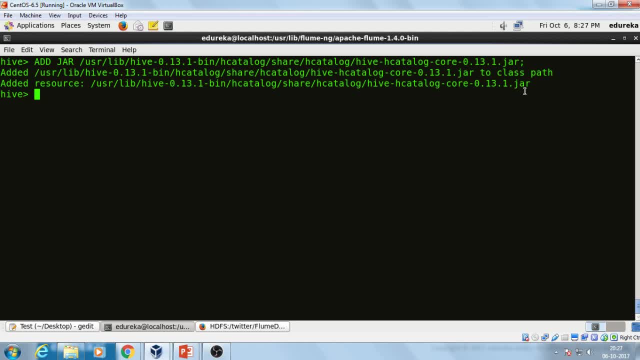 So surd basically means a serializer and deserializer. however, will not get much into what surd is, So you'll get to know more about when we discuss Hive. So basically, I've added my surd here So you can see added resource. 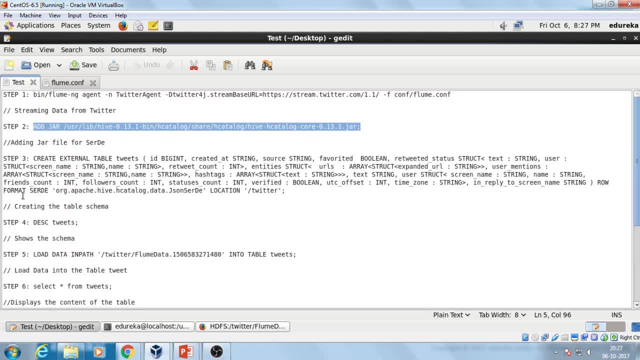 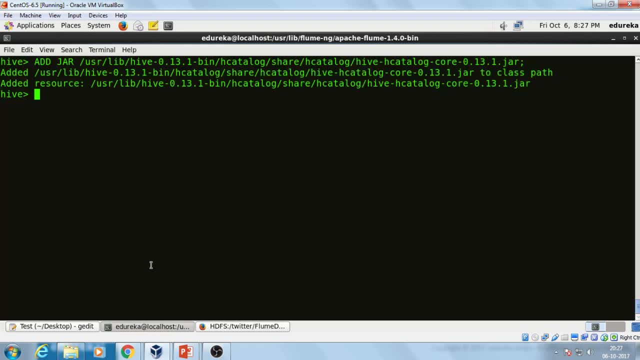 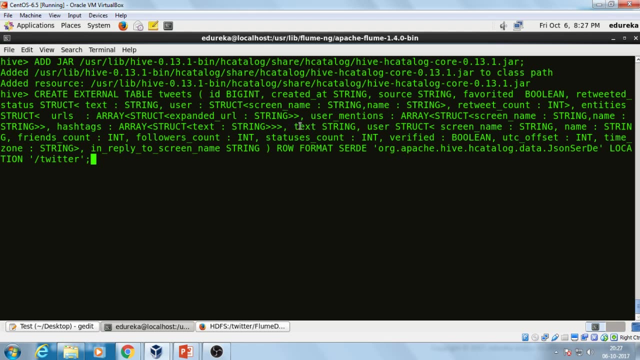 And the next thing that I'm going to do is that I'm going to create A table, So I'll be defining a schema using this command. all right, So I'm pasting, So I'm creating a table called tweets, and I've mentioned the different fields. it will 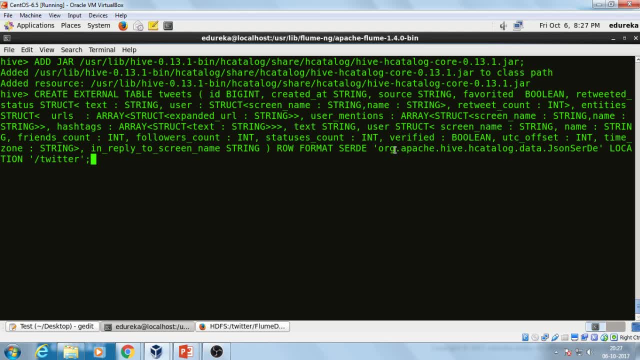 contain, along with the different data types, And I've also mentioned the surd it has. Okay, So we are using hcatalogdatajsonsurd, All right, So I'm just going to run it. Okay, I guess there is one more tweet. 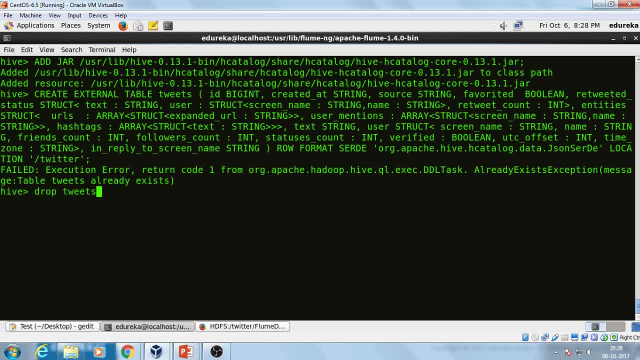 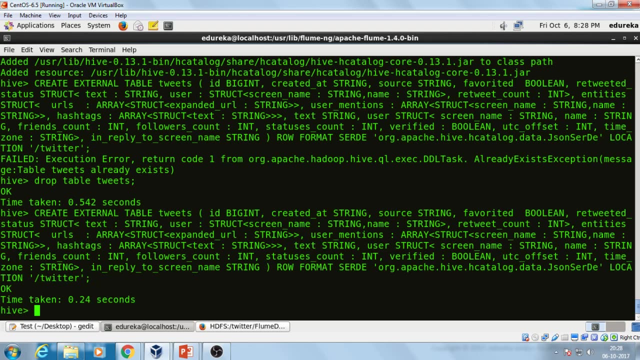 So just to avoid all the confusions, So I'll just delete the earlier table So you can just use drop table tweets. Okay, So we'll run this command again. All right, So it has created a different table called tweets. So if you want to see how this looks like, how the table looks like, so you can just 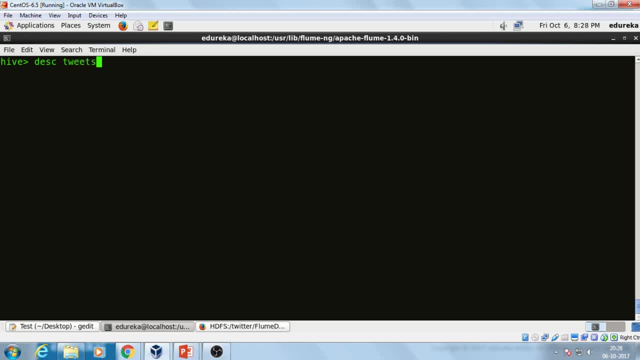 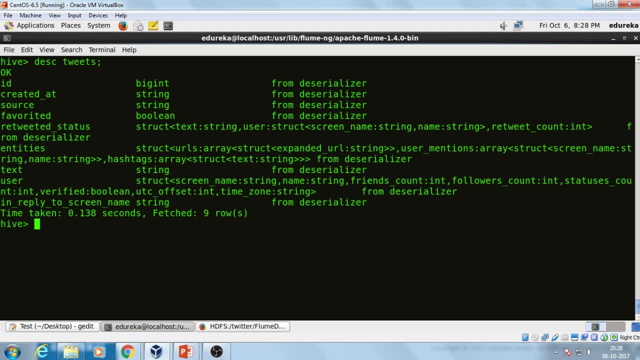 type And I'm going to say describe tweets. All right, So here is what the table looks like And, if you would have noticed, the Hive query language or the Hive queries that I'm running are very much similar to SQL. So if you're already familiar with the SQL language, it is not going to be hard for you. 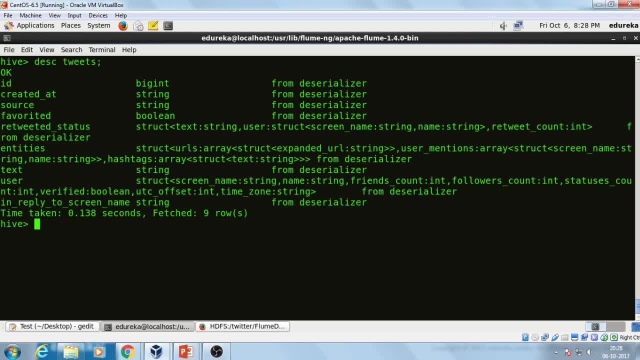 to learn Hive query language. Okay, So this is what the table looks like, And now I have created my table. All I need to do is that I have to get all the data from the Twitter directory in my HDFS and put it in my table. 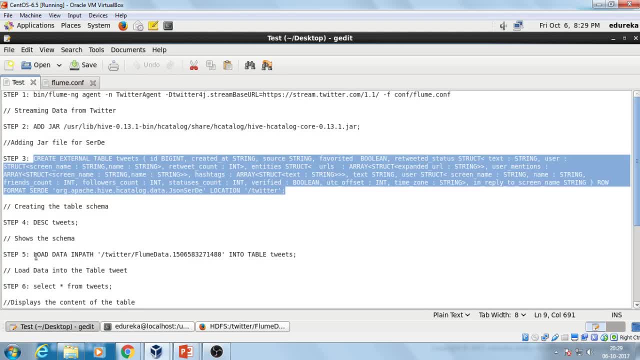 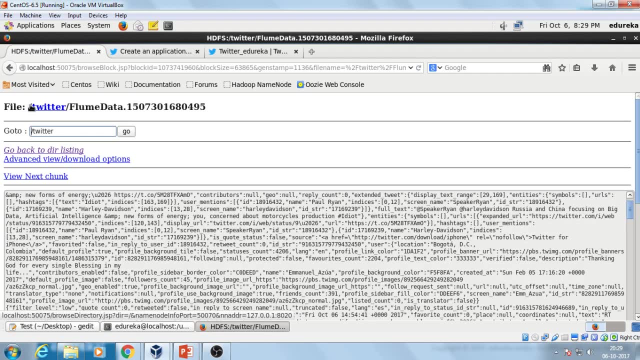 Okay, So for that I'll be using this command. So I have to use this command: load data in path and I have to provide the path in my HDFS. So I will just go and copy the actual path, okay, in the command, because that might be. 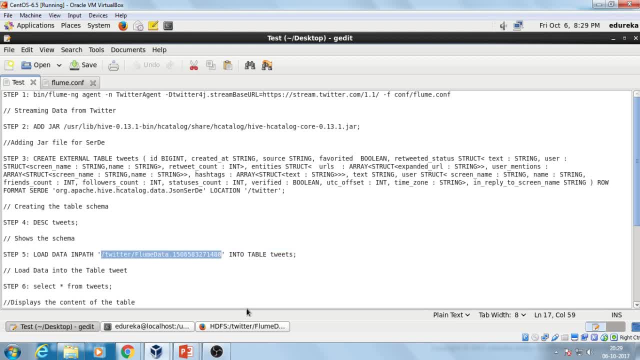 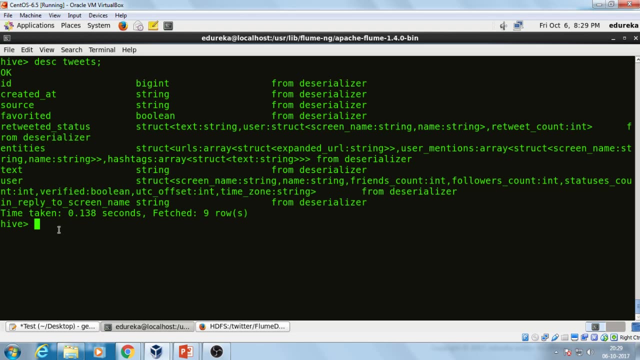 not the correct path here. Okay, So this is the command that we're going to use. That is So. what this command is going to do is that it will get all the data, all the tweets in my Twitter directory, and it is going to dump it in my table. 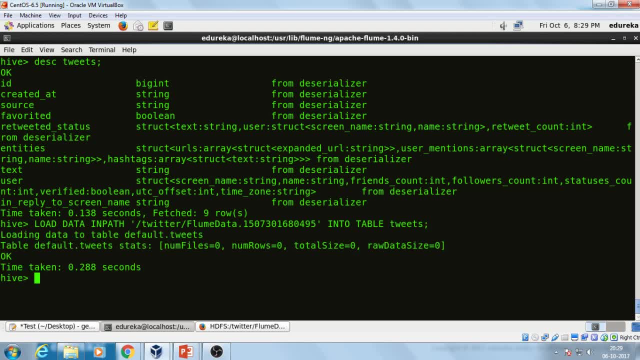 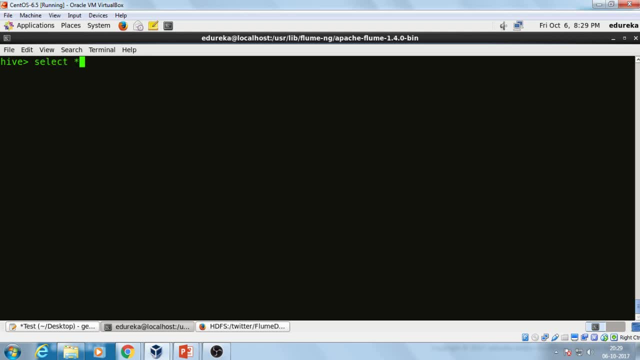 Okay, So it has dumped. So let me just show you how the table looks like now. So you just use select star from the table- name is tweets- and end it with a semicolon, just like how you do in SQL. All right, 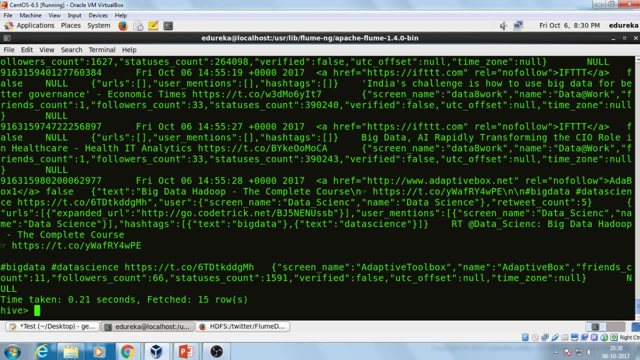 So this is what it looks like. So now I have got fetched my tweets. it is there in my HDFS from HDFS. I have created a table using Hive and then I have got all my tweets into the table. So now I can make some more analysis on it, right? 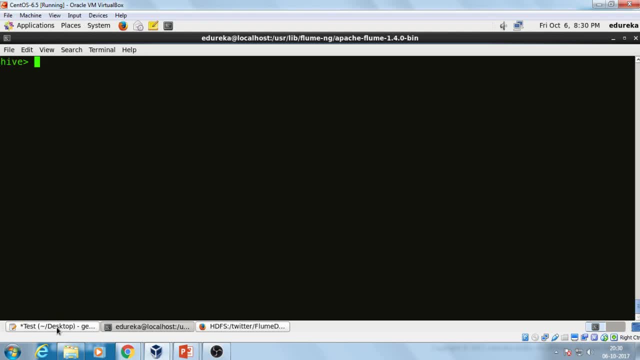 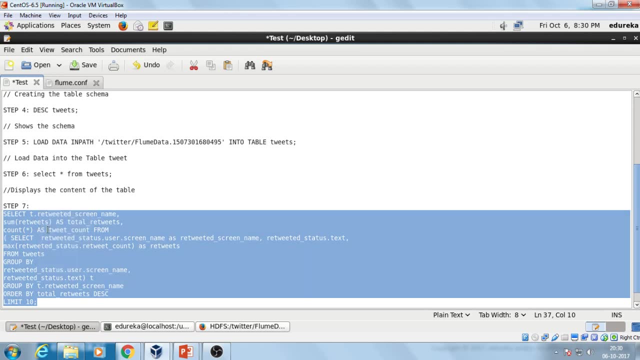 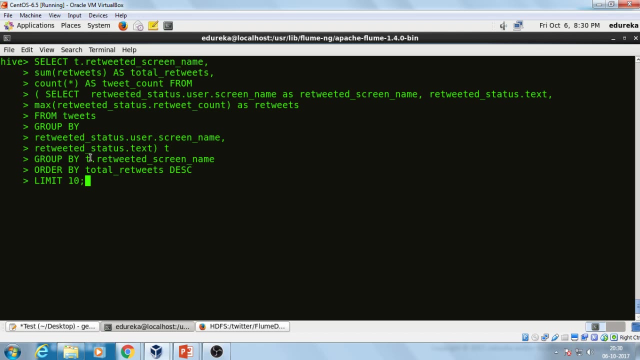 So let me clear the screen and let us do some analysis on it. So for that, we'll be running some Hive queries. Let me tell you what these commands do, Okay, Okay, So here I'm just pasting it. So, basically, we're going to find out what is the activity about big data and Hadoop in. 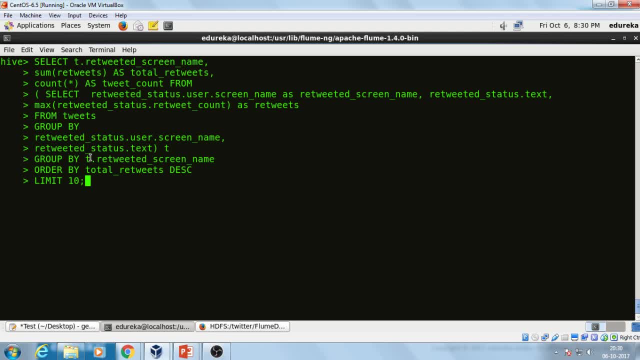 Twitter. So if people are tweeting about it and if there are many retweets on a particular tweet, it means that people are discussing about it. There is a lot of fuss going on about big data and Hadoop right, So this is what we're going to find out. 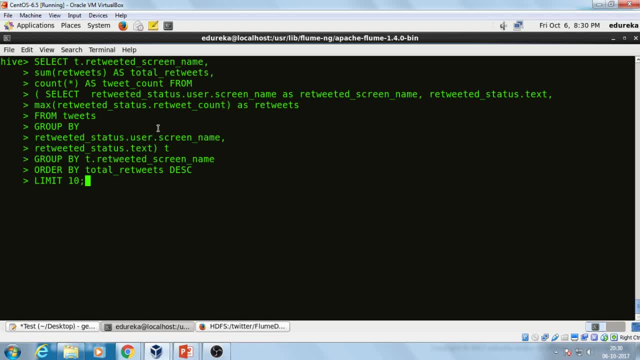 We're going to find out how many tweets, how many retweets on that particular tweet, And then, finally, we're going to find out the top 10 tweets. Okay, So this is what we're going to find out, So the top 10 tweets on big data and Hadoop, and we're going to sort it in descending order. 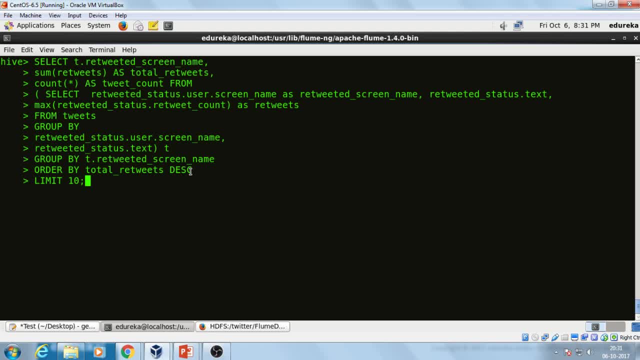 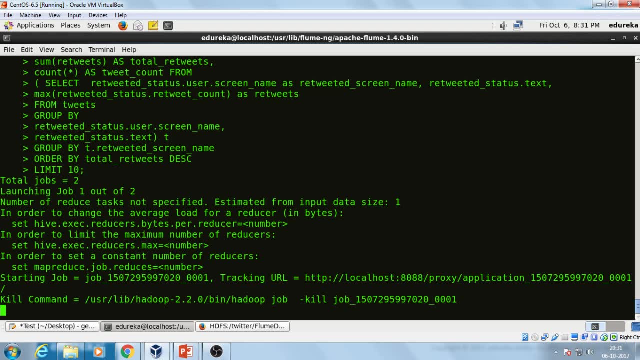 So the most popular tweet about big data and Hadoop will come on top and the rest nine will come in a descending order. okay, So I'm going to run it. So it is launching job one out of two and there are two jobs because we have got a nested. 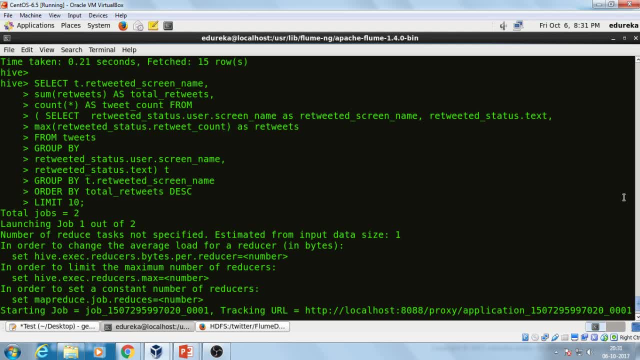 query here. So then, the first thing, it is going to find out whether, what is the username of the person who has made that tweet, whether it has a retweet, And the second job, it is going to find out what is the username of the person who has 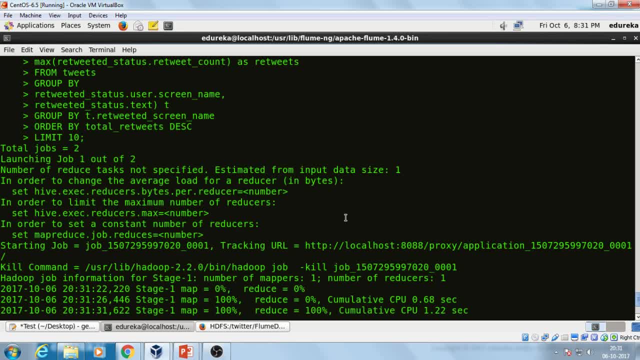 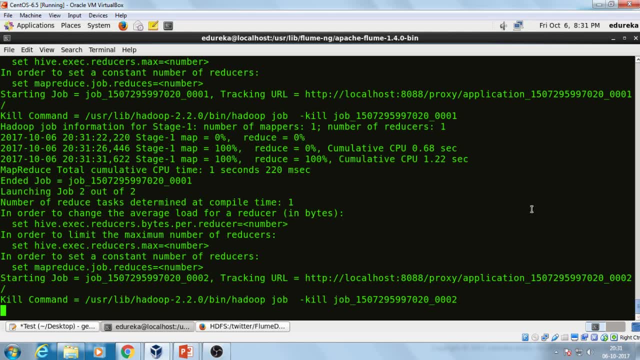 made that tweet whether it has a retweet. So it is going to count how many retweets and all okay. And also let me tell you that it might happen that I'm not going to get top 10, since I didn't. 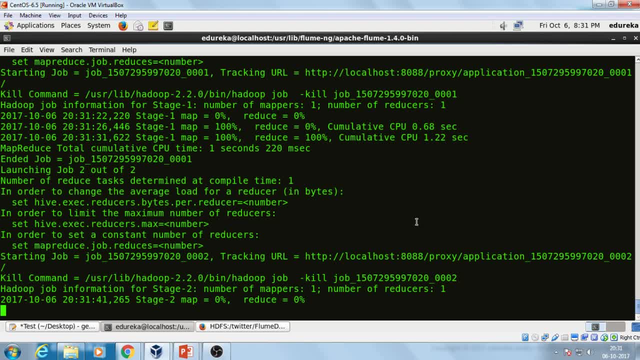 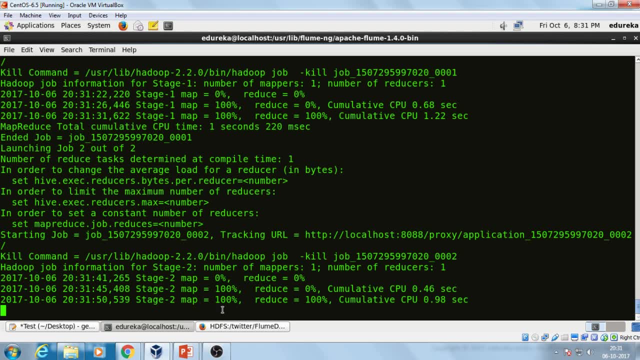 leave my flume longer to fetch all the data, all right, So it might happen that we might not get 10.. And you can see that there is a MapReduce going on, because behind every Hive query there is a MapReduce job running. 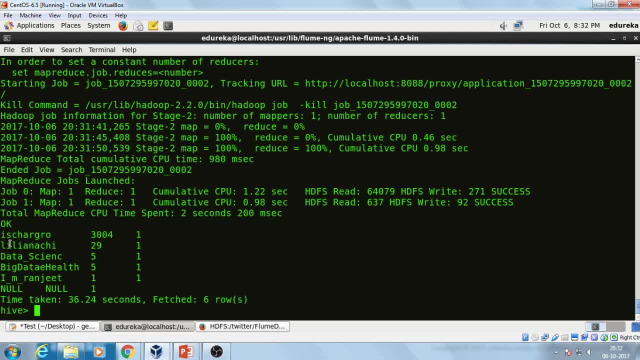 And here we have our result. So here is the username, which is charGrow. So for one of his tweet you have got 3,004 retweets. So definitely you can just make out or you can just tell that there is like a lot of. 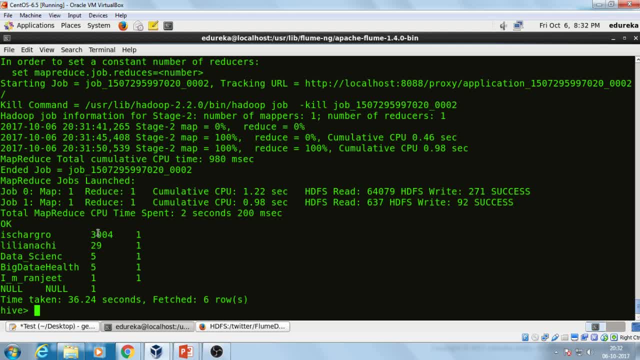 activity going on about Big Data and Hadoop, because if one tweet has got 3,000, more than 3,000 retweets- and I have just left it for just a few seconds, right, So there might be more tweets about it. 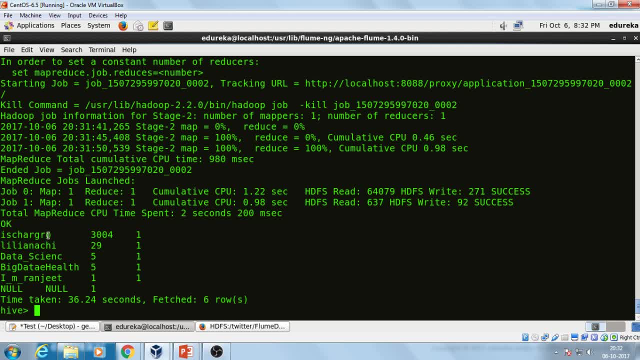 So here is, Since I was telling you we might not get 10, so I've got 1,, 2,, 3,, 4,, 5, and 6,. 1 is null, So we've got six rows, okay. 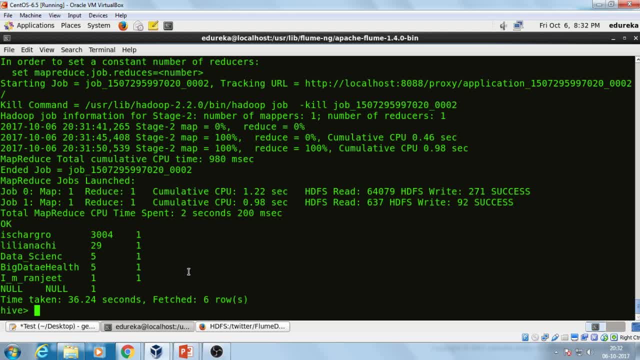 So this is the analysis that we have made. I hope you have enjoyed it. You can also go try it out at your home in your own system if you have Hive and Flume installed. okay, So now let us go back to our presentation. 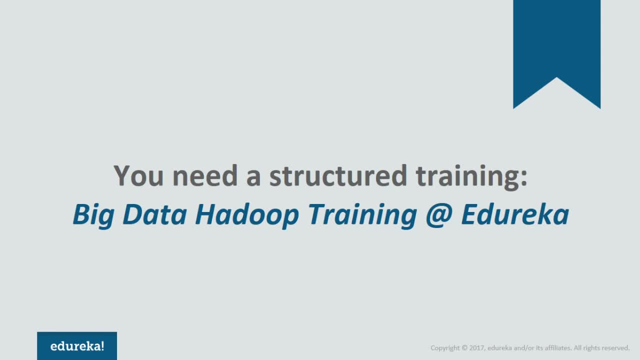 So if you want to learn, I have shown you very interesting things. but if you are interested to learn more about Big Data and Hadoop training and you want to take up it as your career option, let me tell you that you need a structured training for that, because there are a lot. 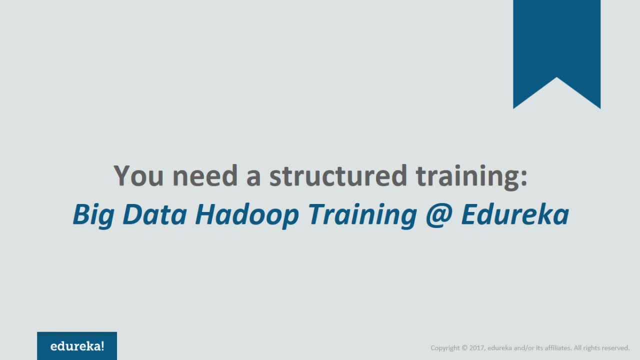 of available content online, and there is a very good chance that you might get lost or you might end up learning just a little and not the entire thing, And that is why we at Edureka have designed a structured training program for you. So let me tell you what this curriculum is all about. 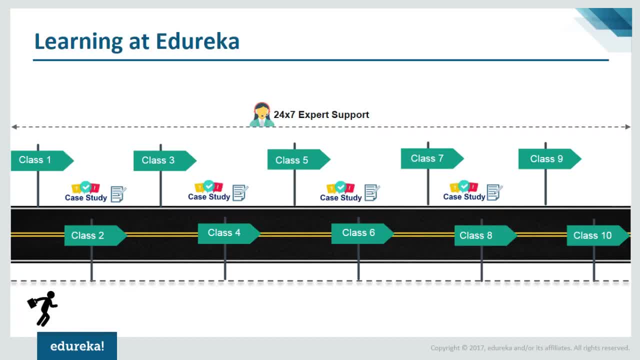 Thank you, Bye-bye. So the Big Data and Hadoop training at Edureka is a five-week of online live instructor-led training class. So in the first class you'll be learning about the introduction to Hadoop, how Hadoop has solved the Big Data problem. 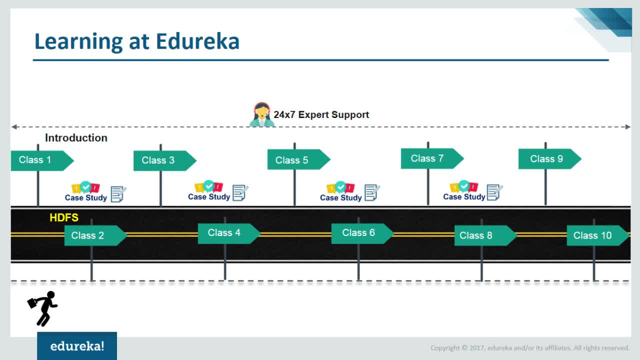 And then in the second class you'll be starting with HDFS, how to set up a Hadoop cluster, a single-node cluster, multi-node cluster, et cetera. And as you move on from the first class to the second class, you will be doing some assignments. 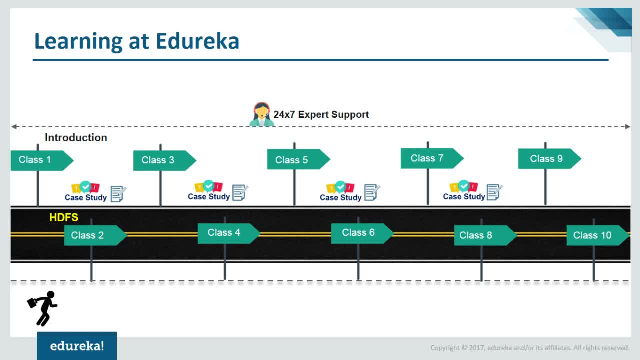 and you'll be studying some case studies, some real-life case studies, And let me tell you that practice is very important, And this is exactly what you will find at Edureka, Because you'll learn all the concepts from anywhere, But it is very important to practice because that is exactly what you're going to be doing. 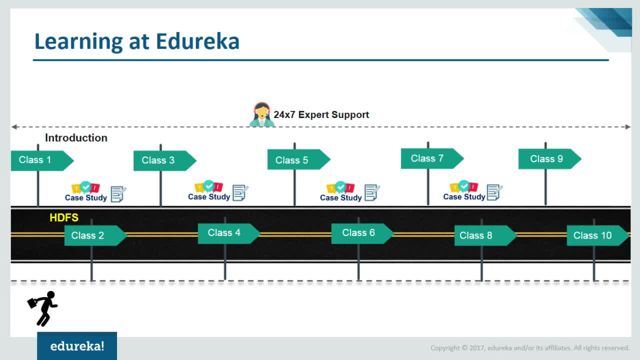 out there in the real world right, And I know it is very hard to find relevant projects online. So you have got case studies and assignment designs on the concept that you have just learned recently in the previous classes, So you'll get a very good practice. 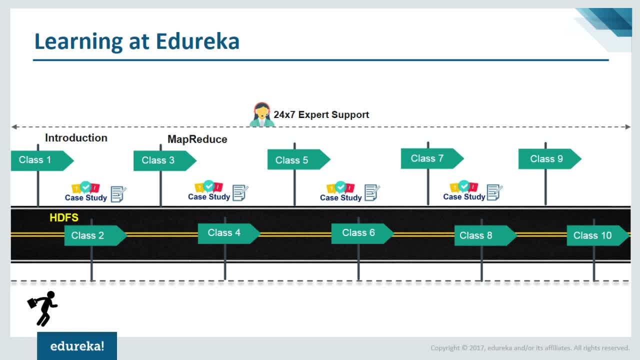 And the third class will be a very, very good practice. Bye-bye, Bye-bye, Bye-bye. In the third class, you'll be starting with MapReduce. In the fourth class, you'll learn some more advanced MapReduce concepts. 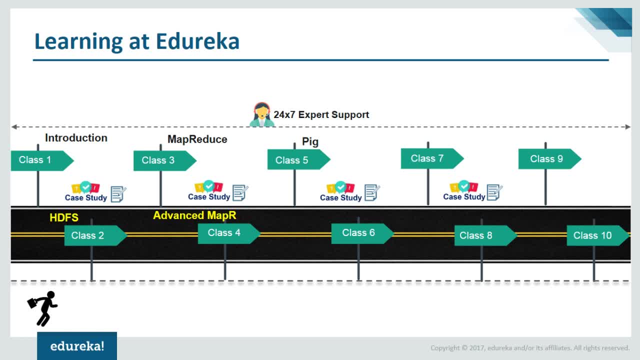 Okay, in the class five you'll be starting with Pig, which is a scripting tool, as I told you. Then in the class six you'll be learning about Hive. So here you'll get a detail about what Asserte is and how it works and everything about Hive. 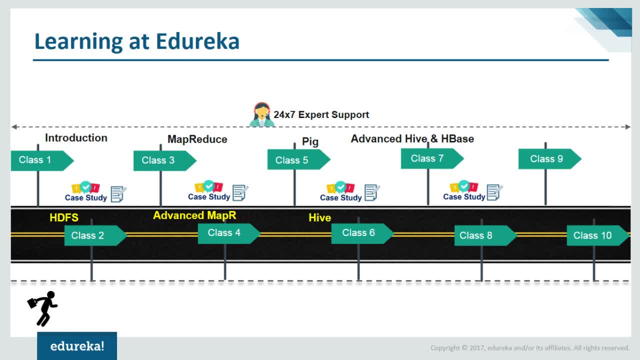 and some advanced concepts of Hive also in the seventh class, And you'll be starting with an introduction to HBase in the seventh class. HBase is a NoSQL database that is highly used in industries nowadays. You'll learn more advanced HBase concepts in the eighth class. 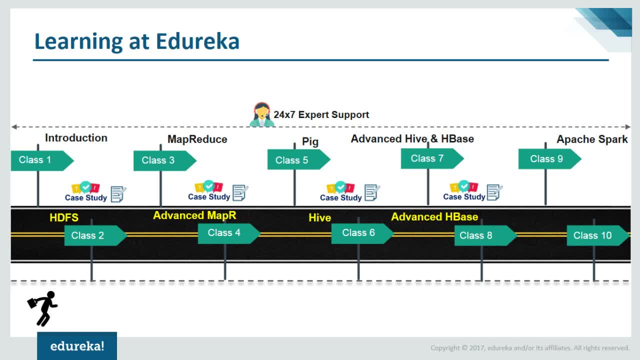 In the ninth class, Apache Spark, which is used to process real-time data. Here you'll be learning about all the different components of Apache: Spark. Apache, like the Spark SQL, then Spark MLlib and all other related concept. resilient- distributed. 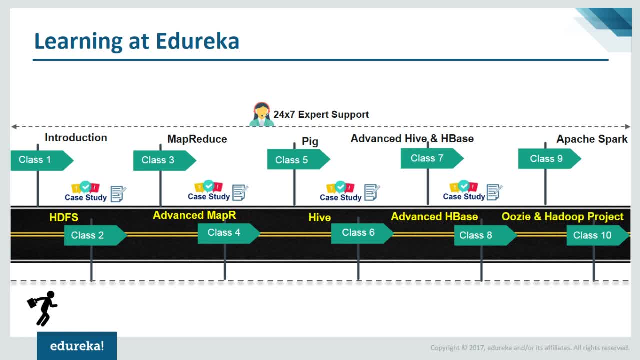 databases, et cetera. And in the tenth class, finally, you'll learn scheduling with Uzi and you'll be commencing with your Hadoop project. Okay, So, after you have completed all the classes, When you've completed your assignments and project, you will be Big Data and Hadoop certified. 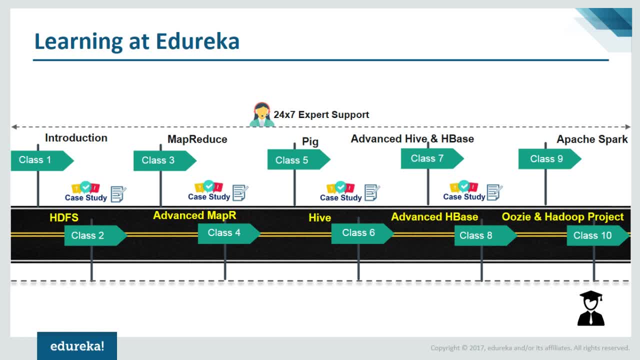 by Edureka, And let me tell you that the certificate that you're going to get is a verifiable certificate and you can put it up on your LinkedIn profile, which is, I think, very much beneficial for you because it will give you a very good exposure to your future employers. 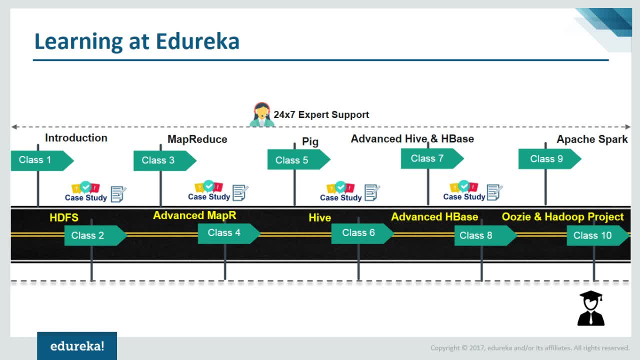 And apart from that, Edureka certification also holds a very good industrial recognition. We have a lot of clients that you might have heard of, like Visa Ford, So they trust on us And so definitely you know that if these companies are trusting on us, definitely it has got. 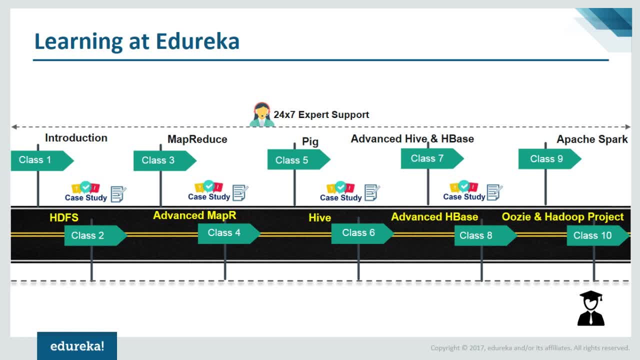 a very good industrial recognition. And, in case that, if you're wondering that, what if you ever get stuck in between your assignments or projects? so don't worry For that. we at Edureka have a 24-7 team of expert who is going to help you and guide. 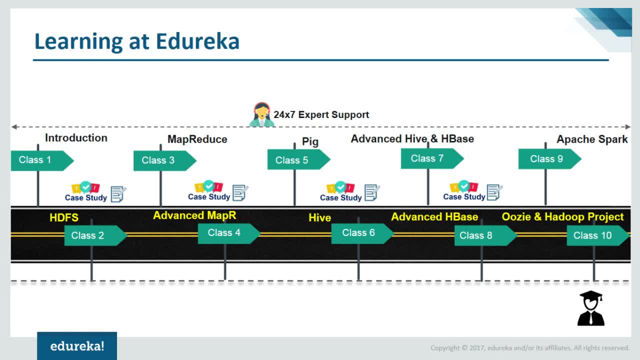 you in case you come across any problem, maybe at 3 am in the morning or at any time of the day, And they will get back to you instantly and solve your problem. And apart from that, there are more benefits to enroll with Edureka. 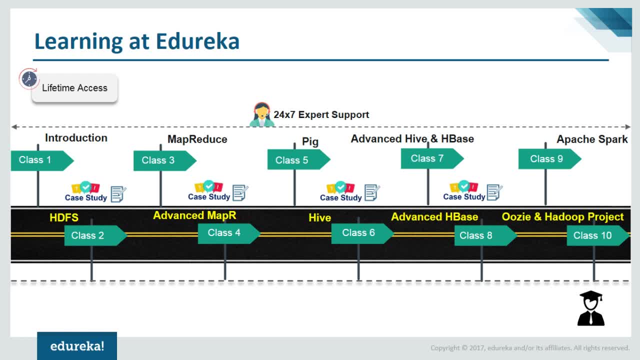 First, you'll get a lifetime access to your Elemis, So your Elemis will contain all the required study materials that you'll be needing in order to get trained on big data and Hadoop, and you'll have a lifetime access to you. 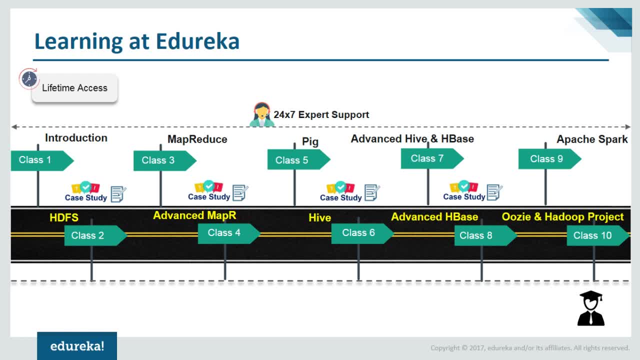 And meaning that, even if you have completed the course and you still want to revisit after some time, to go through all the concepts, you can still do that, even if Hadoop has come up with a new version. And that's what we're going to do. 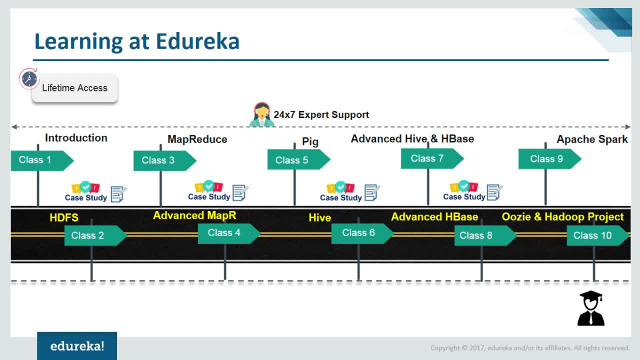 And we have upgraded our course according to that. you can still go and access the newly upgraded course, even if you have studied the older version, And even if you're going for an interview and you want to go through all the concepts again after a year or so, you will have access to it for a lifetime. 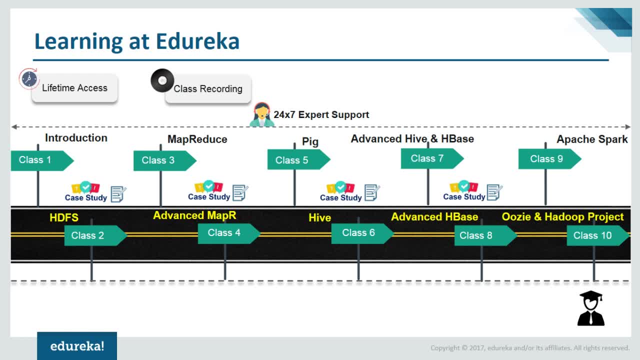 Apart from that, your Elemis will also contain a class recording after the completion of each of the class, So you can go through it again And even if you want to re-attend another class with our industry experts, we're going to instruct you during the sessions. 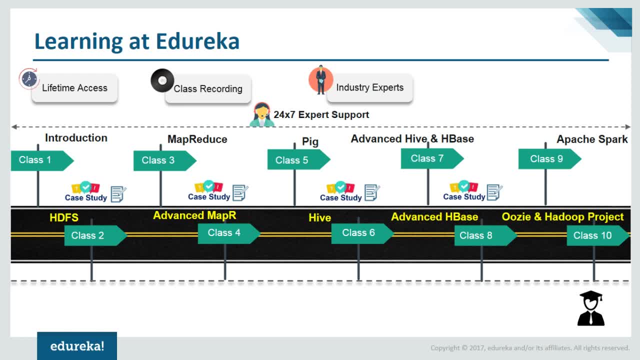 You can still do that without any extra cost And the industry experts essentially are the early birds in this particular technology and they are the subject matter experts, So they have essentially 12 to 15 years of industry experience and they will be sharing. 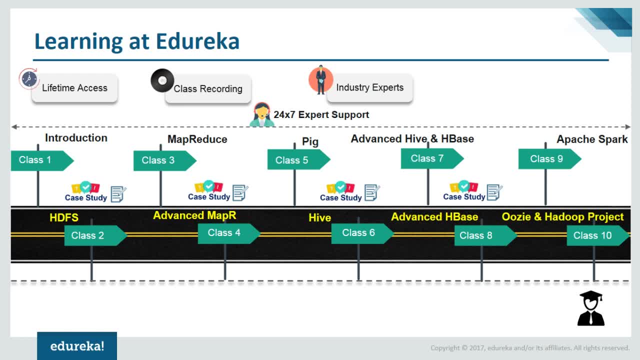 real-life case studies with you, which are actually ongoing projects in different companies, So definitely, you'll get a taste of what it is like to be a big data professional even before you become one. And, finally, there are multiple projects to choose from, and this is very important because 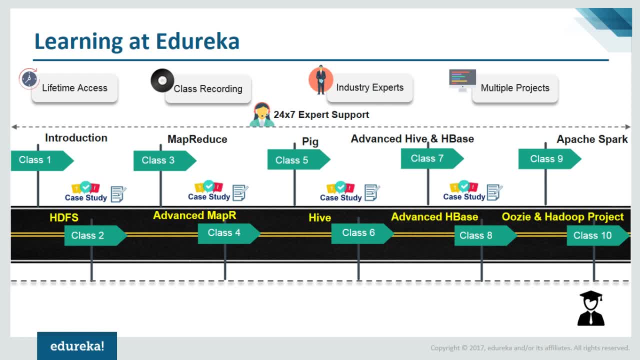 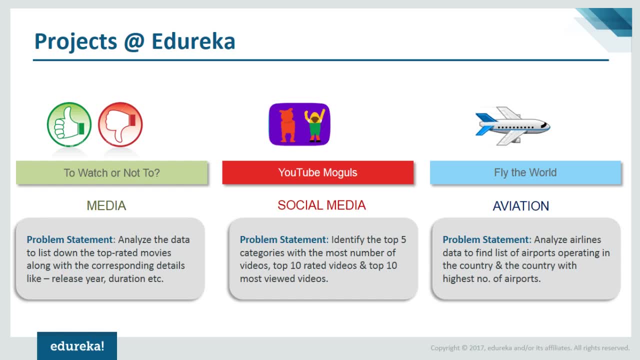 you need to put in a lot of effort, You need to practice, You need to put all the concepts that you've learned into use. So let me just tell you what are the different projects that we have at Edureka. So the first one is related to media. 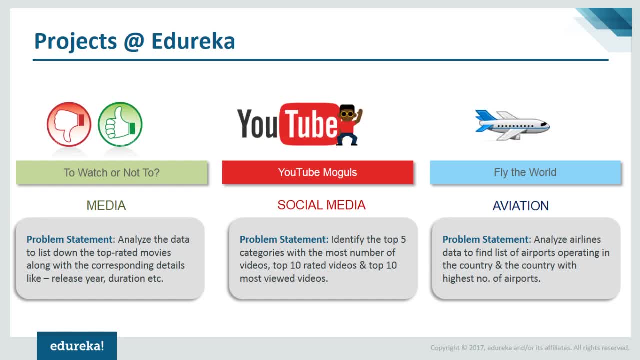 So this here will be designing a system very close to IMDB. So here you'll be finding out what are the most top-rated movies, so that you can recommend it to the users, And also you'll be finding out some more corresponding details with that movie, like the release. 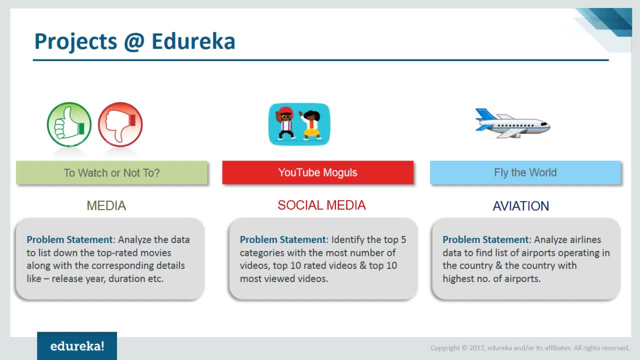 year duration, et cetera. The second one is for our fellow YouTubers here, the YouTube moguls. So one to be the moguls in YouTube. So for them you'll be analyzing to find out and identify which are the top five categories. 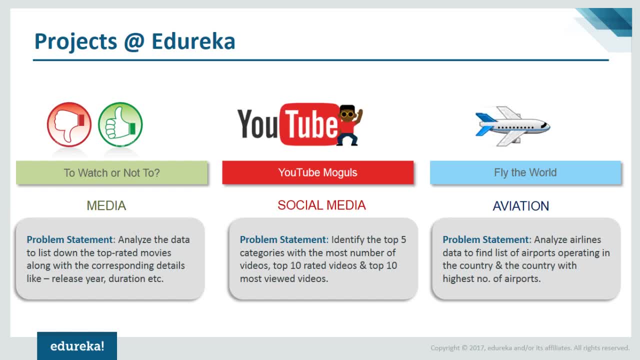 that they can make video on in order to make their channel and make their videos more popular. Okay, So you'll be finding the top five categories and what are the top videos- the most rated and the most viewed videos in each of the categories. 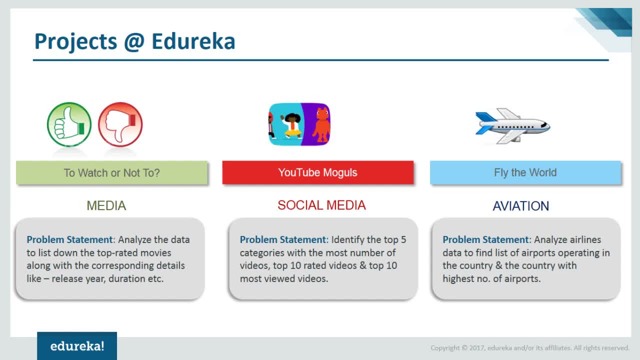 The next one is related to aviation. So here you'll be, pretending that you're working as an analyst for a newly like airline company. So they have given you a job, They have given you the task that you need to. I need to find out that. which are the? 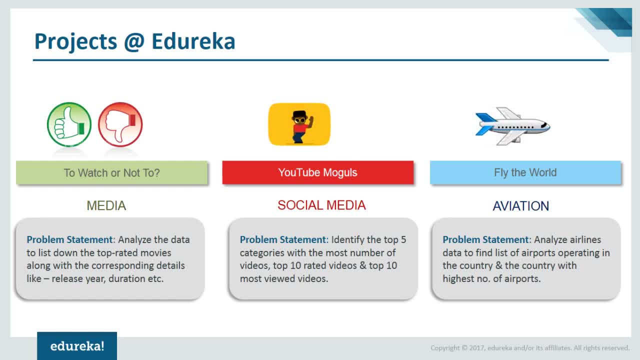 most busiest airport? which country has the most busiest airport, so that they can station their newly crafted airplanes in those airports? So you'll be analyzing the airlines data to find the list of the operating airports in a country and which country has the highest number of airports. 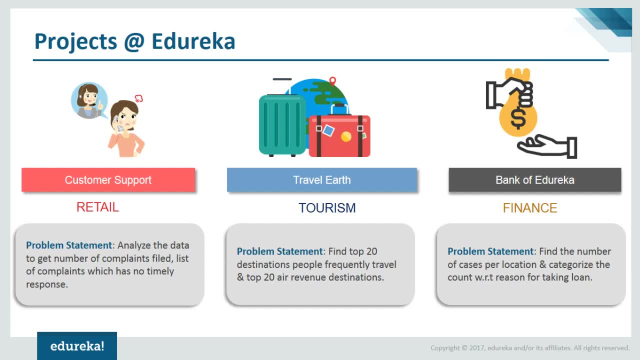 Then the next one is related to retail. So this one is related to customer support, which I think is very important because you need to keep your customers happy, right? So here You'll be designing organization data to analyze, and here you'll be finding out that what are? 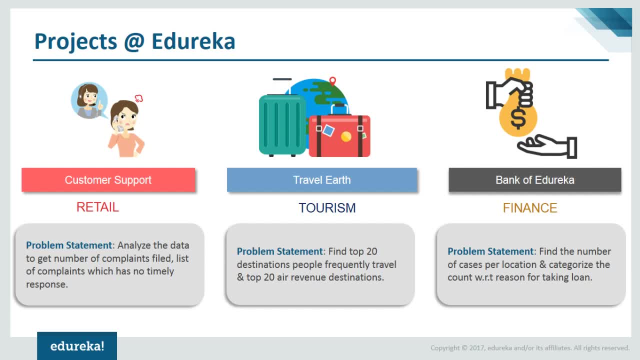 the total numbers of complaints filed and which are the complaints that did not have any timely response, so that you can put them up in the top priority list and they would be taken care of at the earliest, because you don't want unhappy customers. Then their next one is related to tourism, the travel earth. 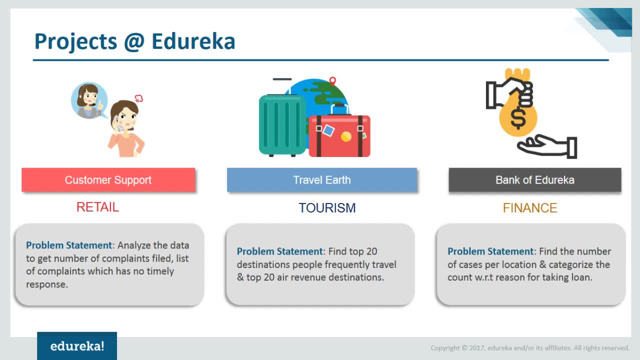 So here you'll be designing a system very close to TripAdvisor. I'm very sure that you've heard about TripAdvisor. So here You'll be Using people, some popular holiday destinations. so you'll be given a travel data set to find out which are the most popular, most traveled places so that it can recommend it to the. 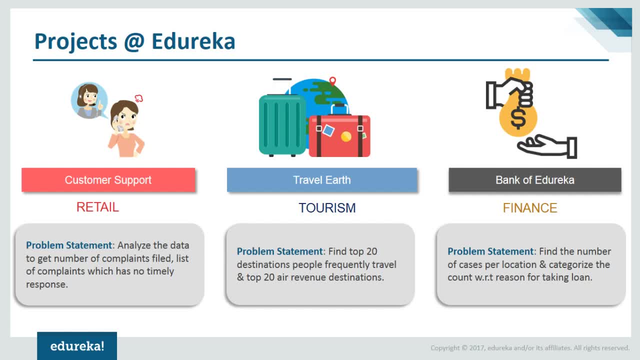 users as the popular destination that they should travel to. You'll also be finding out some top 20 air revenue destinations and some more analysis on it. And then there is the imaginary bank of Edureka. This is related to finance, So here you'll be finding out on categorizing different loans according to the reasons given. 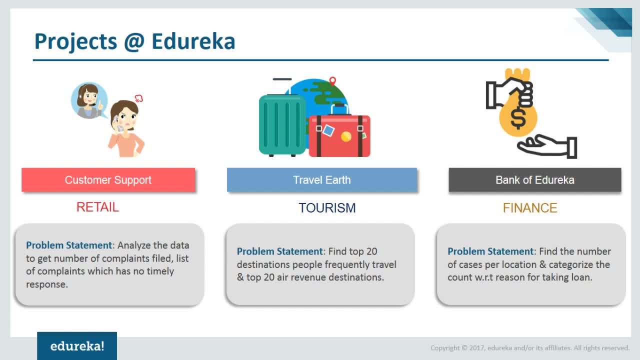 So definitely, You know, here you'll be like categorizing, like how many car loans, home loans, personal loans, etc. So these are just the six of the projects that I'm showing you. There are many others to choose from. 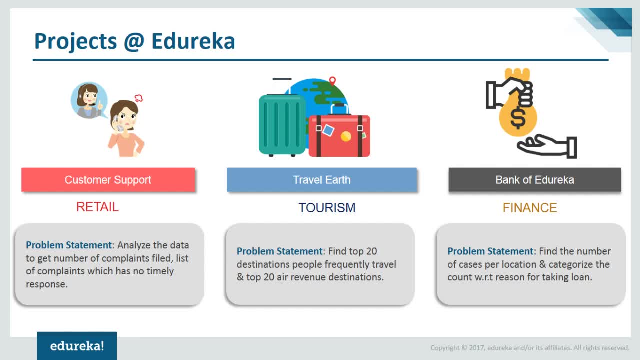 You can choose to complete any one, some of them, or even, if you want, you can choose to complete all of them if it looks interesting to you. Okay, And don't worry, you'll be guided by our support team and our experts in order to complete. 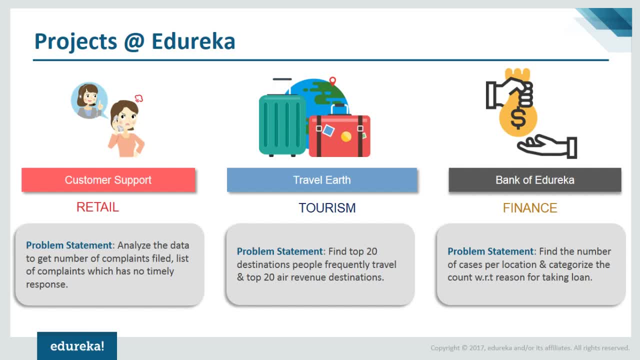 your project And if you also see we've got a wide variety of projects related to every domain. So the six that we saw have, like, different domains: media, social media, aviation. there is travel, finance, retail, et cetera. right, 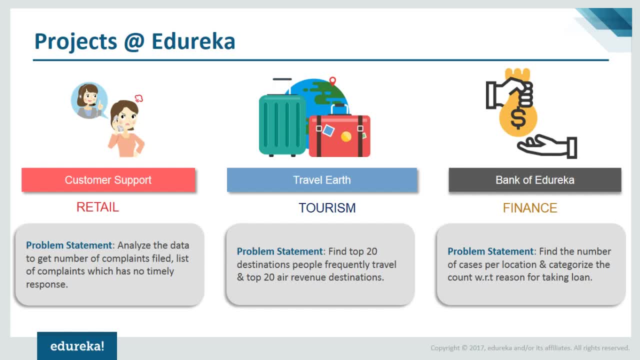 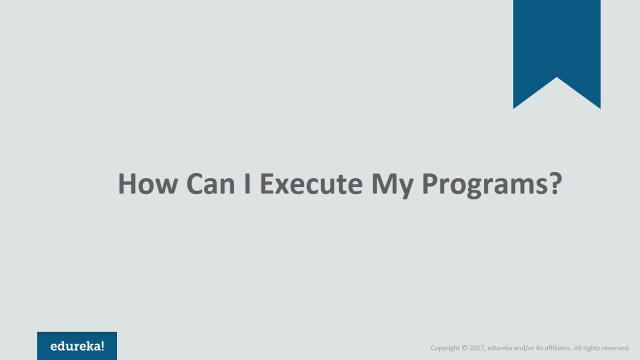 So these are very interesting projects that you can choose from. if you choose to learn it from Edureka and enroll the Big Data and Hadoop course, And if you're thinking that, okay, I've chosen my project, how can I just execute it? 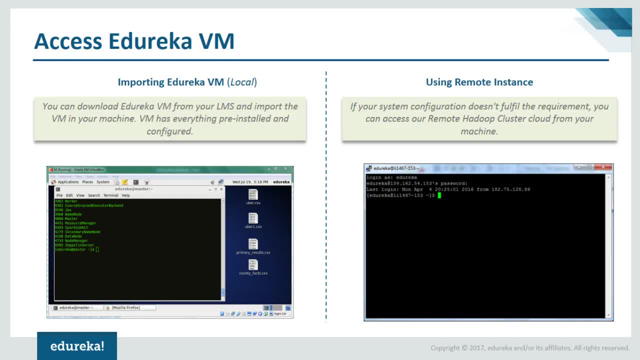 Where will I execute all my programs? So don't worry. So once you enroll with Edureka, you will be given a virtual machine that will have all the softwares pre-installed for you in order to run all your programs and projects on. 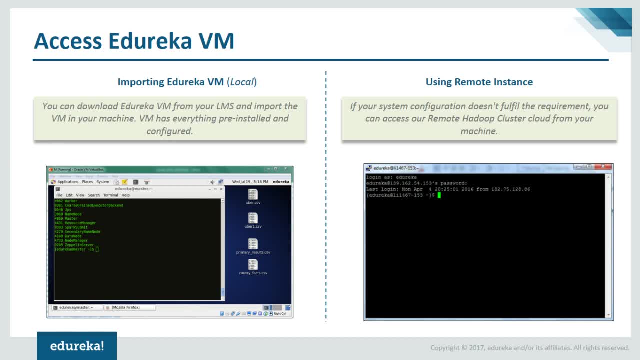 Okay, And even if your system, let's say, does not comply with the configurations that is required in order to install the VM and run the VM, don't worry, you can still use the remote instance. So you'll be able to. so you'll be given an access to the remote Hadoop cluster. 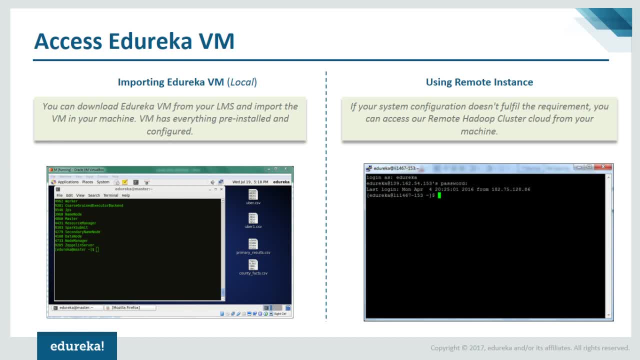 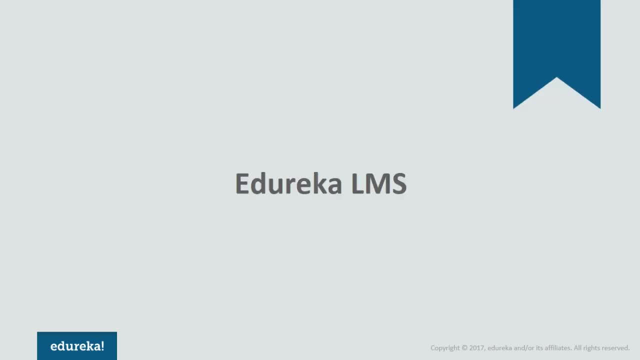 So you can access that. This will also have all the softwares pre-installed. All right, So then let me just show you the Edureka Elemis, what your Elemis is going to look like, how everything is stored there, Okay. 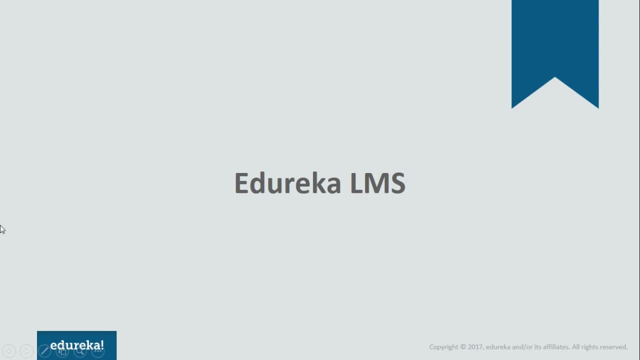 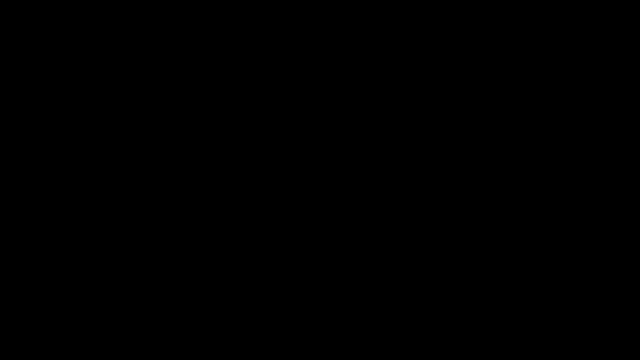 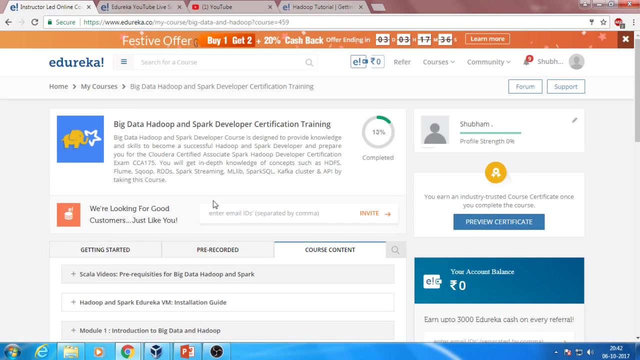 So let me just open the. okay, so I hope you're able to see my screen. You're able to see the Elemis, right? So I want some confirmation. All right, I guess you're able to see my screen. So here is what your Elemis is going to look like. 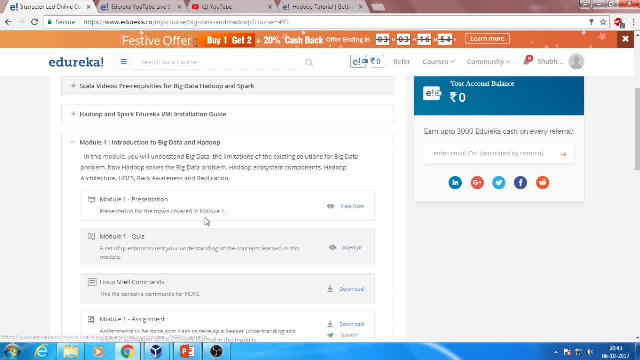 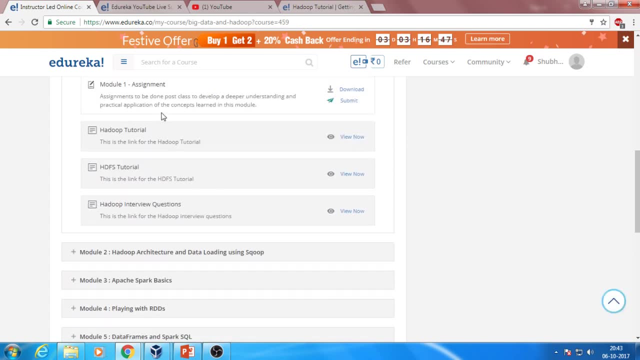 It will have different modules. So if you click on here so you can find all the presentation quizzes, assignments, tutorial and all the interview questions, So it will contain all the documents that is required for you to understand Big Data and Hadoop. 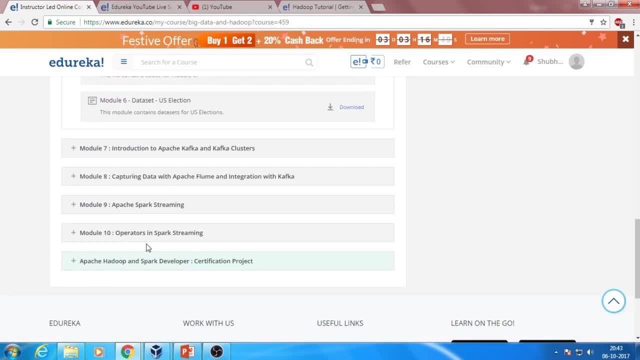 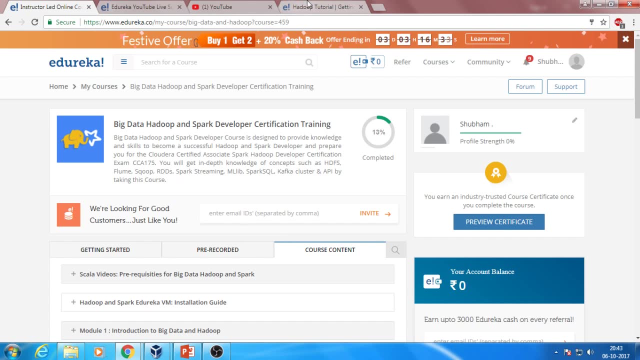 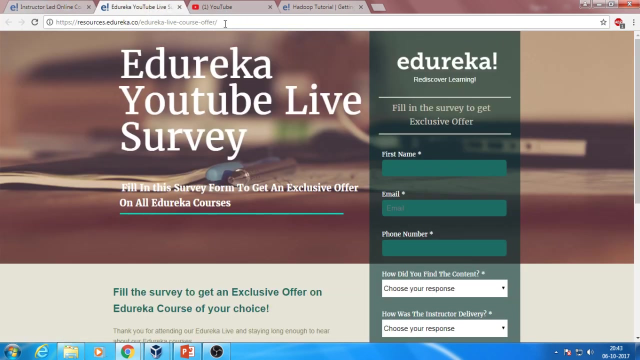 And you will have a lifetime access to it, So you can just have all the details about all the different modules here. Okay, And then there is something for you all, So I will be sharing this link. So this is basically a link to a survey form. 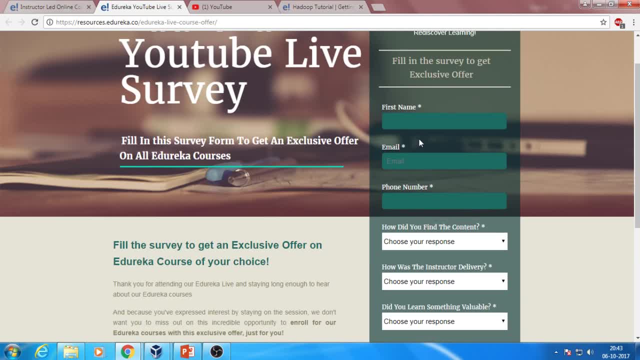 This is going to look like this, So please fill it up so that we can improve our content better, And for you, this is also beneficial. Let me tell you how, because it will help you to avail some exclusive offers if you ever choose to purchase any course from Edureka. 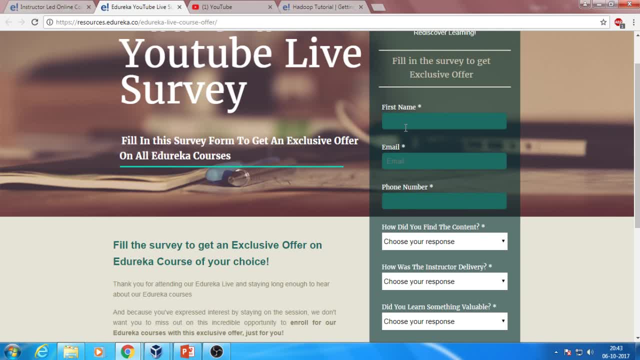 So make sure that you fill up this survey form, So make sure you provide your correct email address, correct phone number and your name so that we can get back to you and provide you with the exclusive offers. And, of course, it will help us to give you a better learning experience as well. 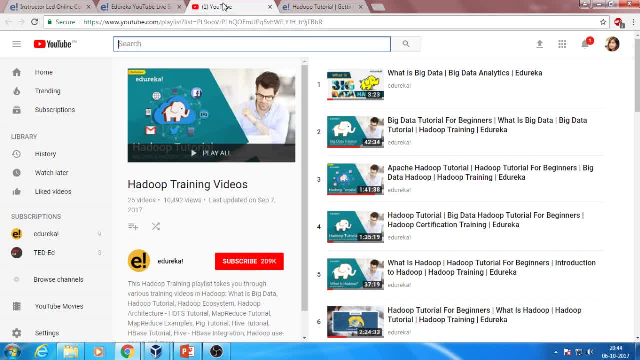 Okay, And here you can find. if you want to learn more about Big Data and Hadoop, we have got some tutorial videos on our Edureka channel on YouTube So you can go through this playlist. So it has got different videos- How to get started. 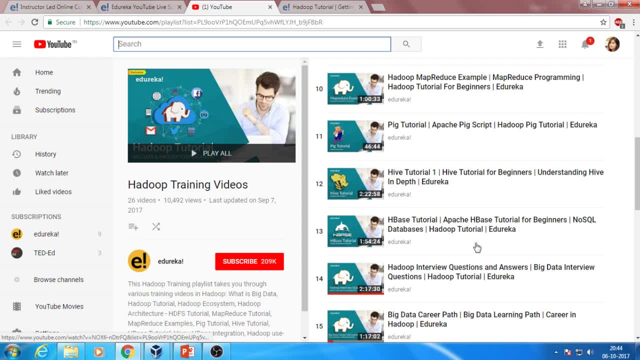 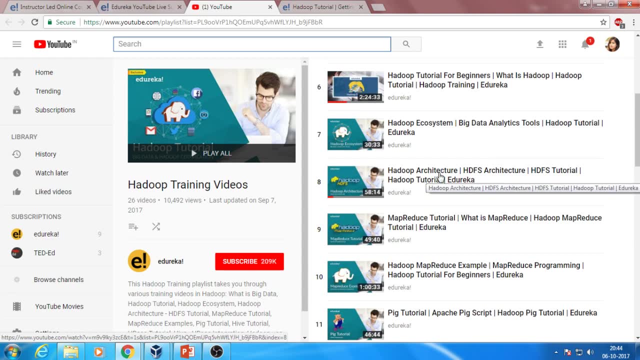 How to get started. How to get started: We have a lot of videos on Hadoop, on Hive, on Pig and all other Hadoop ecosystem tools, on basic Big Data and Hadoop, So you can go through all the videos and make sure that you click that like button, if it. 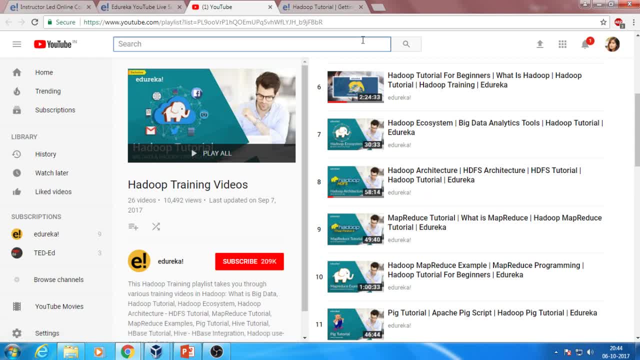 is able to help you. if you learn something, Okay, And also if you want to know if we are coming up with more videos, make sure that you click on the bell icon on the video, So it will give you notifications every time we upload any video which is going to be. 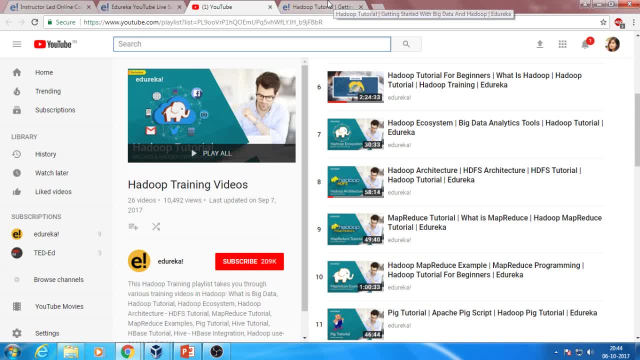 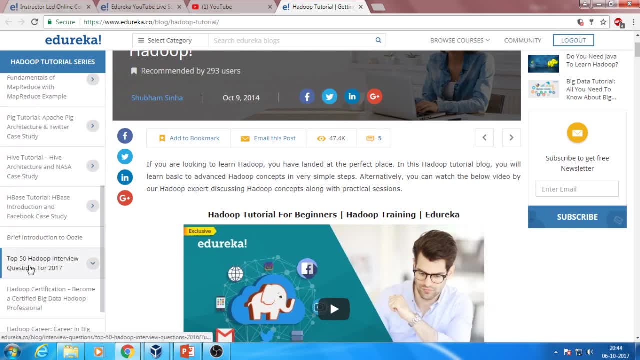 very much beneficial for you, since you get to learn a lot, Okay, And you can also go through our blog blog series on Hadoop. So there are many blogs on Hadoop that you can go through. if you are fond of reading, I'm very sure that you're going to have a very good reading experience. This is 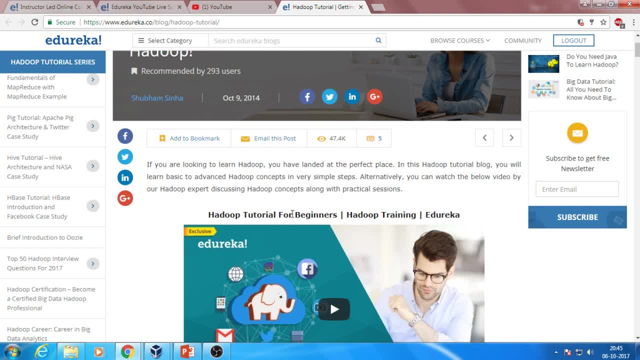 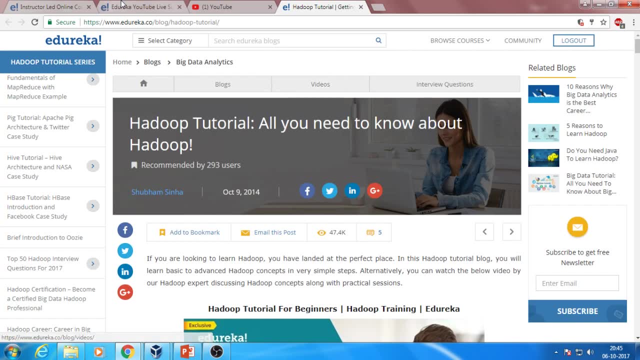 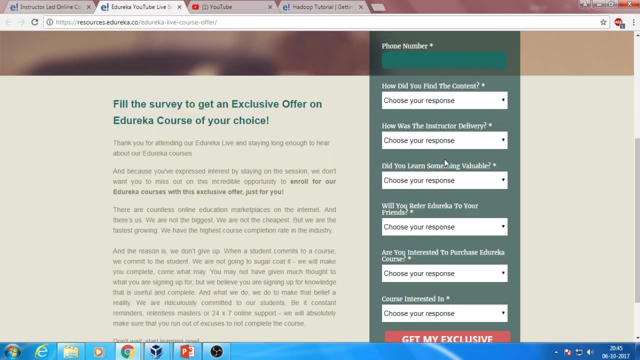 written in plain English, very understandable. Okay, so make sure you go through our YouTube and our blog channel as well. And also please- I will tell you guys again- please fill up this survey form. This will be beneficial for both of us- a symbiosis relationship, right? So you'll get an. 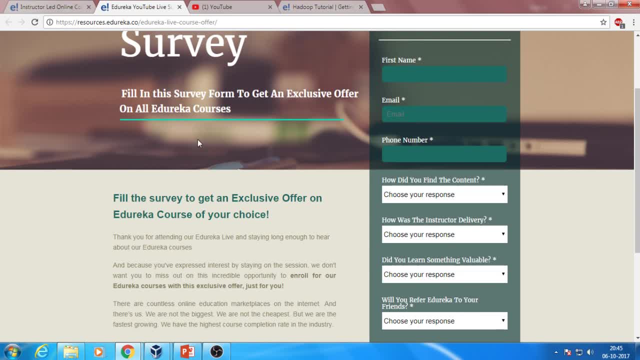 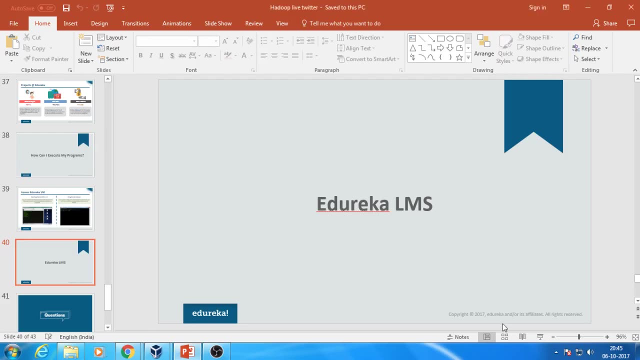 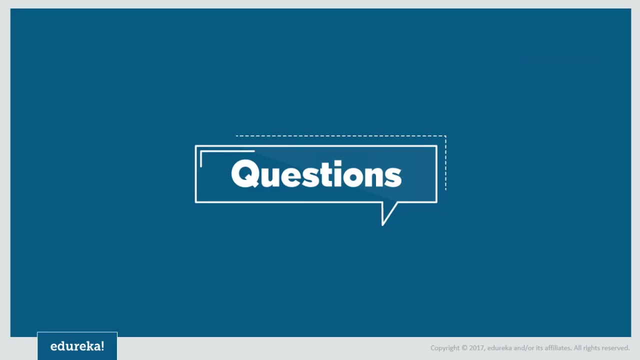 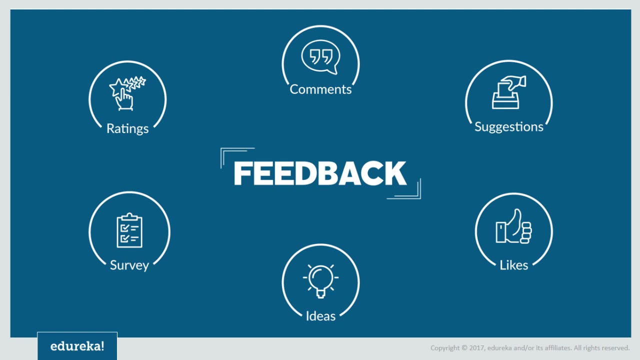 exclusive offer and we'll get to understand how can we make a better learning experience for you. All right, so you can leave your questions on the chat box and also feedbacks, So make sure that you fill up that survey form. Also, make sure to like this video if you have enjoyed learning.